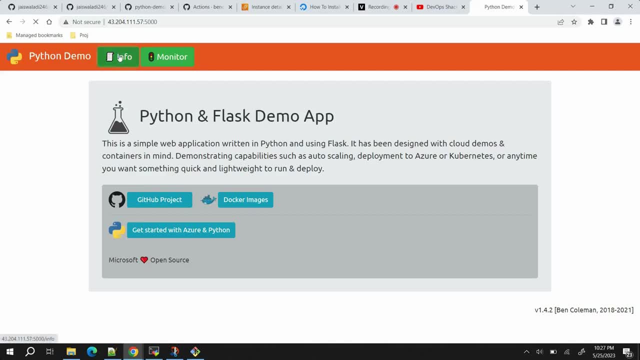 this application is having, and this is the application, So let me show you how it works. If I click on info, then it will give info about this application: what are the things used, and all Okay. then again we have this monitor option, which shows whatever background running processes. 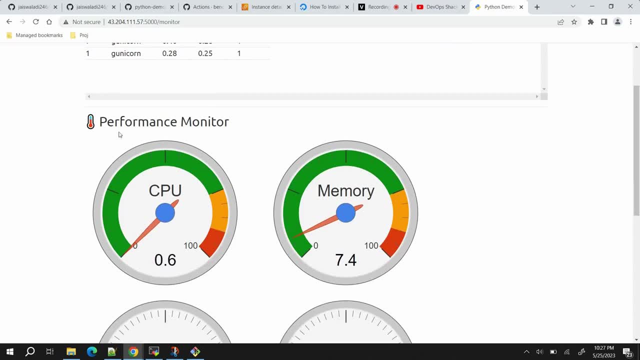 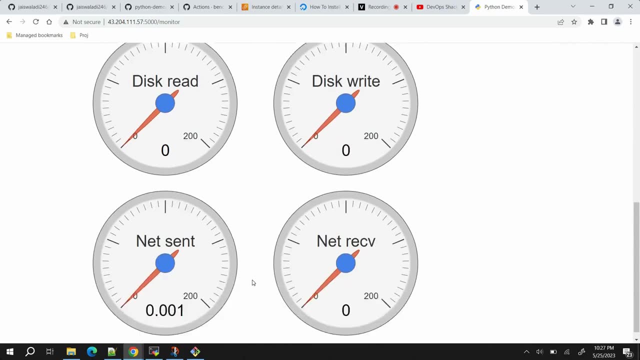 are there and like how much memory they are consuming, how much CPU time. Same thing, performance monitor inside performance monitor can be seen: Okay, these values, they deviate like, they deviate little bit. Okay, and they will give you like proper time, proper like. 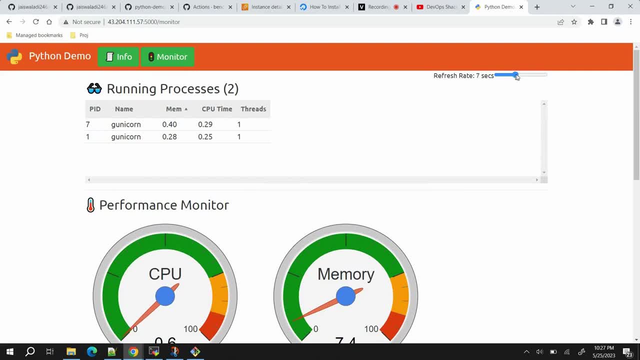 monitoring things. Okay, also, you can make this. there is an option to refresh the page, which you can increase or decrease. So if I keep on two seconds, it will like every two seconds these things will be getting updated and those things will be shared to us, Okay. Okay, now let's have 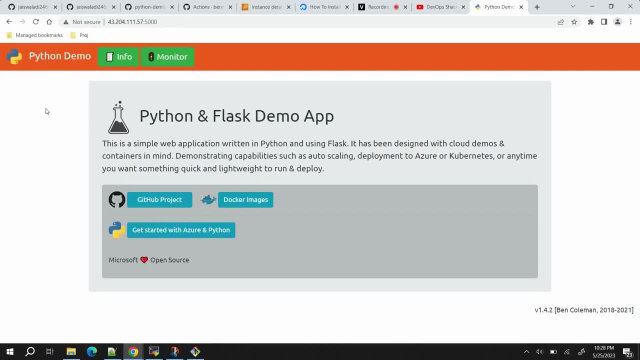 a proper conversation about this project, because always I share the repository to you, which is what I want you to do. I'll be sharing a repository, but that won't be mine, Okay, because in my repository I have done so many changes to make this application work, and that's what I want you. 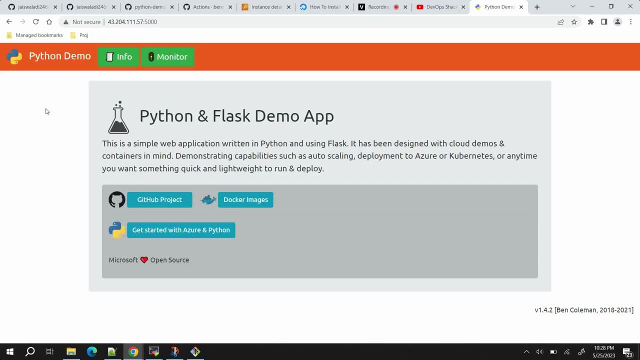 to do, because I just, at the end of the day, I just want you people to learn and understand everything. Okay, so in this video, everything I will show you, like how to make this project work, how to make this project run properly, Okay, but since I have already made the changes in my 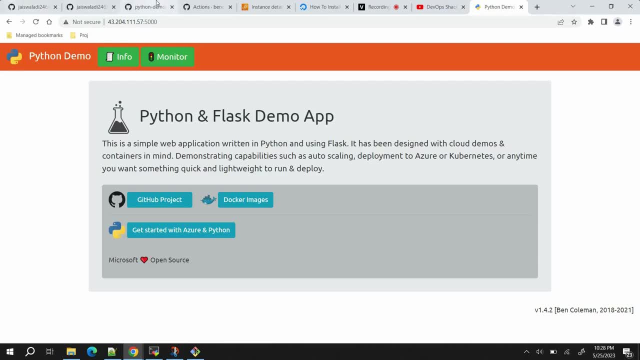 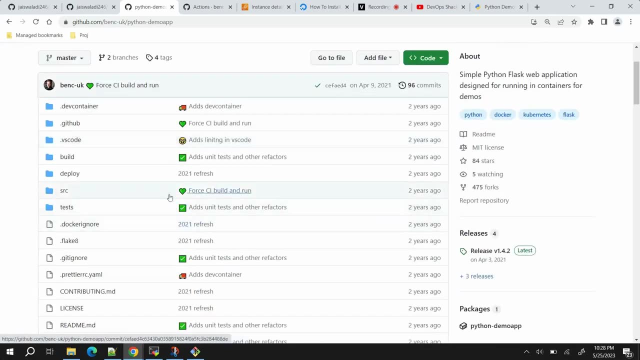 repository to make this project up and running, So I'll be sharing you The original original repository from where I have like forked it. Okay, so if you like to start working with this repository, you won't be able to run, Okay, so what? whatever things is required to 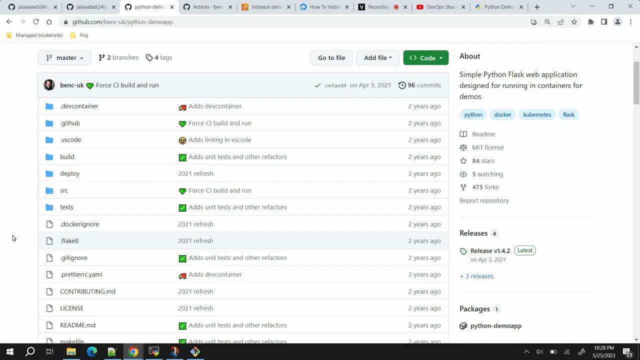 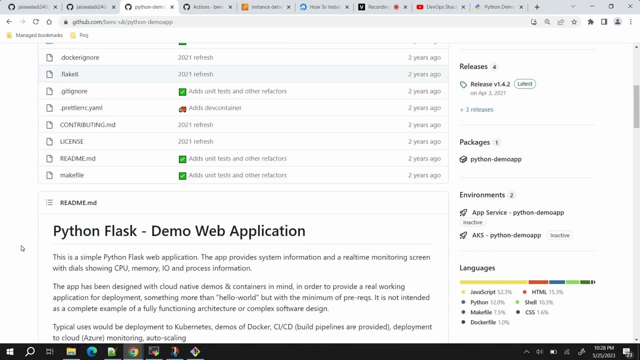 make this project able to build and run. I will inform you, I will show you in this video, also side by side, even though, like, I have just started building for the first time the Python web application. but I learned a lot of things because I was trying to fix things. fix it, Okay same. 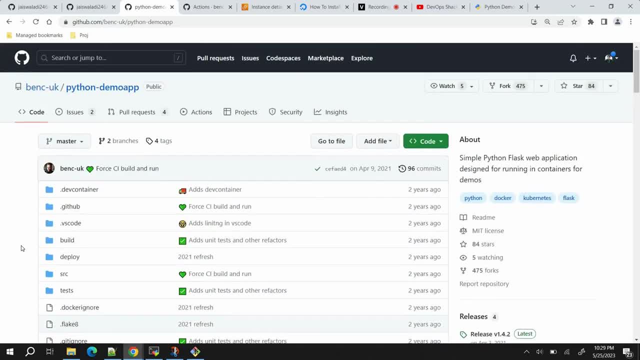 things, and that's what exactly I want you to do. Okay, so I will you just make sure to watch this video till end, because everything I will explain you how this application is working, how we will be able to build this application. Okay, because if you directly just clone this and start running, 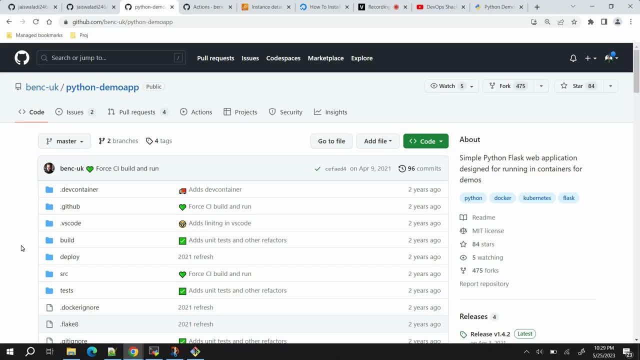 the commands that I do, it will fail. you won't be able to like, create docker container and docker image. It won't work like that, Okay. so I just want that you should learn, then you should implement it, and for that you need to watch the video. 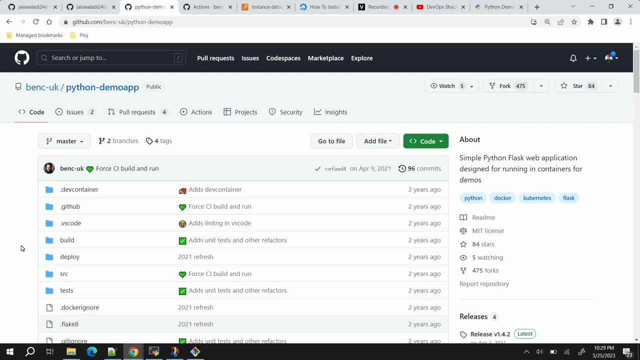 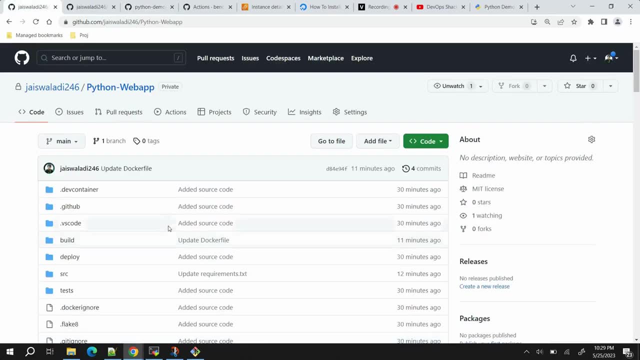 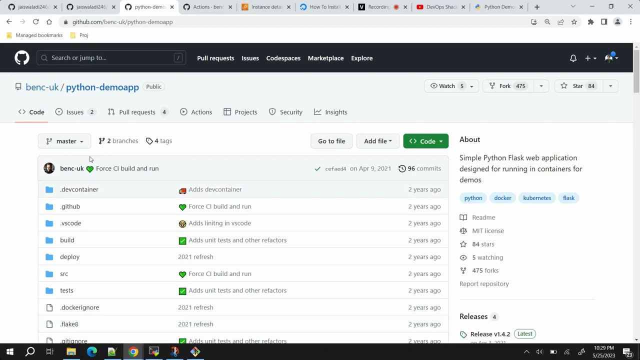 to understand how to make this application work properly. Okay, so I hope you understand, because I'm not literally, I'm not joking. see, this is my repository. I have just made some changes inside it And that is why it is able to getting deployed and it is running now. okay, but this is the main. 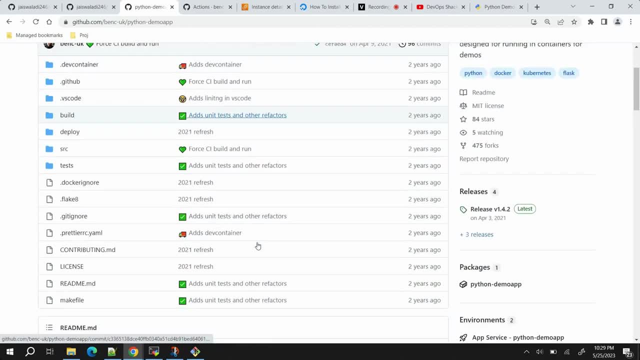 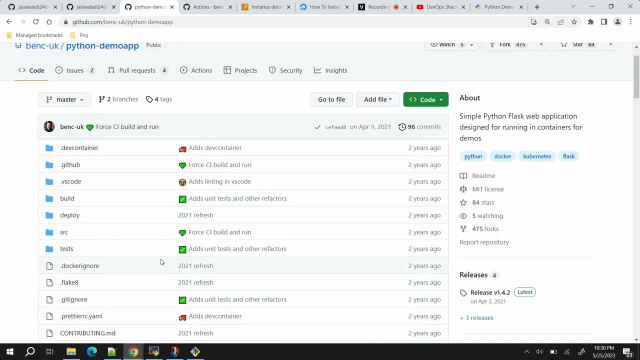 person's repository, who's I have, like cloned. So if you just clone it and run it on your system, it won't be able to. the reason because, first of all, it's two years old and there are so many packages you need to update. and another thing, like you need to understand how to update things in python application, in case. 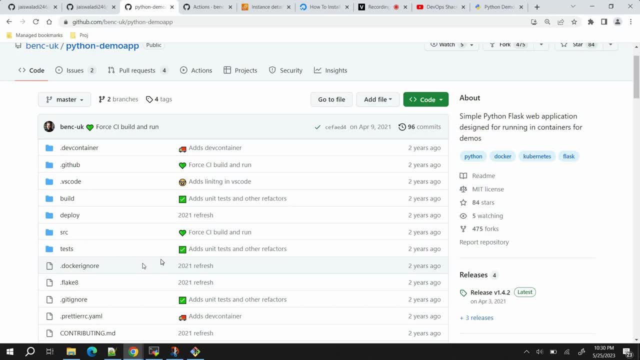 you have already worked it, you might be able to know, but if you have not, then you won't be able to do that, okay, so i just want watch the video, understand what i, whatever i am sharing, and then start building the application from this repository. okay, and then even you will feel very happy that. 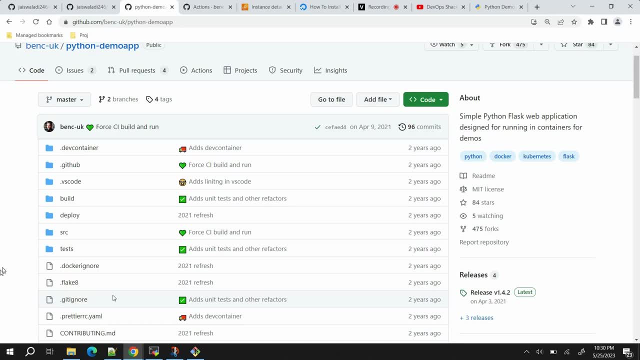 you have fixed it and you understood this python application so that in future, if any application comes to you, you will be able to understand as well as build it. okay, this is like. i know, like i'm talking a little bit philosophy here, but at the end of the day, i just want you people also to 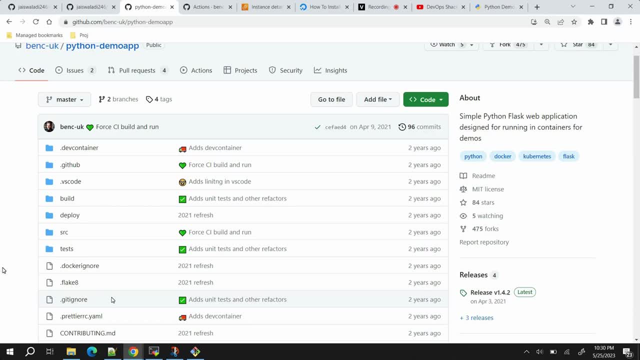 learn and do hard work as much i i do, okay. as much i am benefiting from working hard, you should also get benefited. okay, and see, it's not here that i'm charging any money to you, so i'm just like taking like 30-40 minutes of yours. that also will be reduced once you speed up the video, okay. 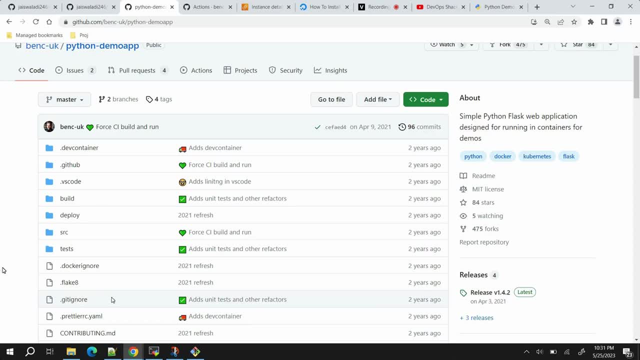 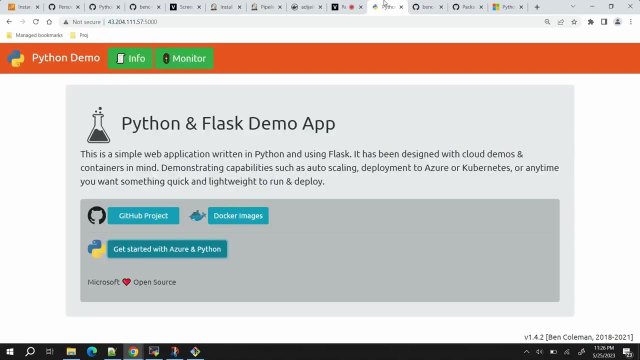 okay, so just watch the video. it will benefit me as well as you. okay, okay. so now let's start the implementation and make sure you understand, step by step, everything. i will tell you, explain you every single thing. okay, so let's start. okay, team. one more thing that i wanted to share that since 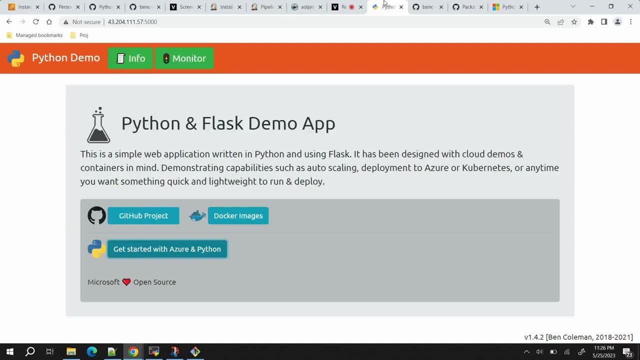 you know like for me, it is very important that we should grow in audience or subscribers, because this is part time and for me to continue a proper way, i like i really need a good audience to watch my videos and i will see you in the next video. bye, bye. 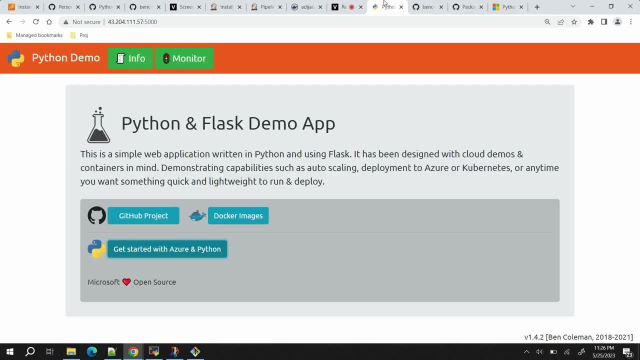 my videos and literally learn everything from it. okay, so if you are watching and if you find these videos useful for you or if you are learning something from them, then i would really request you share them over linkedin in your post, and you can even tag me. i'll be happy to reply anything. 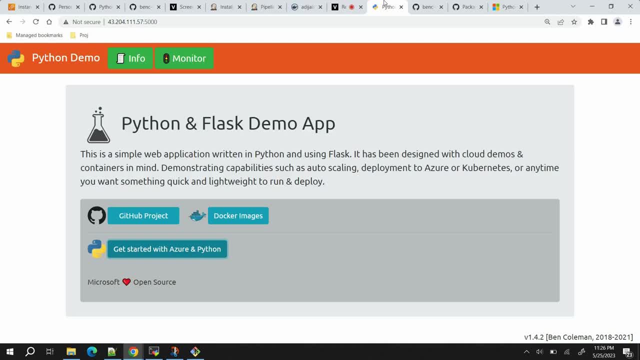 you want, okay, also, like, if you are having any queries, any suggestions, any ideas, you can just ping me over instagram or linkedin. i'm available, okay, but mostly i'll be available after like six, because before six it's like my office hours. so, yeah, really, i would really appreciate if you could, if you could share my video so that. 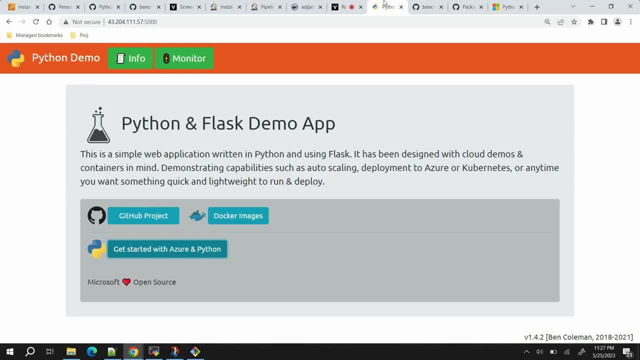 at least some more audience i can get, and i can keep continue like making such videos for you, okay, so really i would appreciate that. okay, now let's come to the main video. okay, team. so now coming to the project, let me explain you how this project is basically, how we can build it. okay, 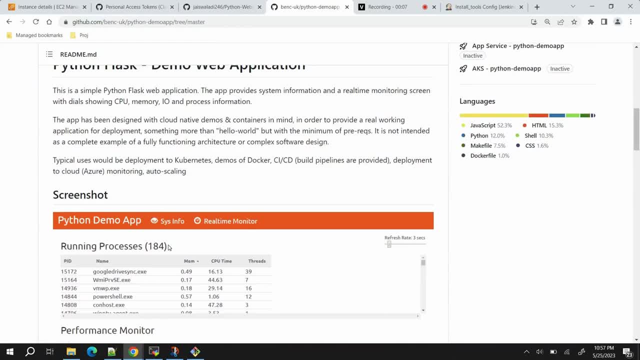 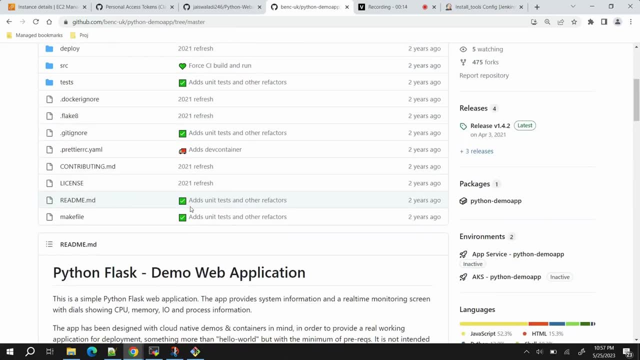 so this is the main structure of the project and if i scroll down here is like make file, which is most important part of the project as of now. basically, first of all, you need to know what is make file. okay, make file is a script sort of thing inside which we define certain rules like what this rule will do, what this rule will do for. 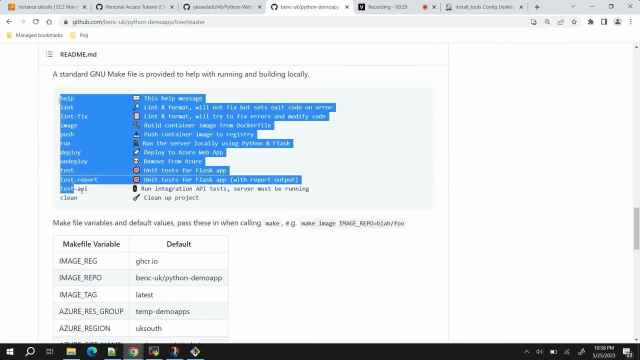 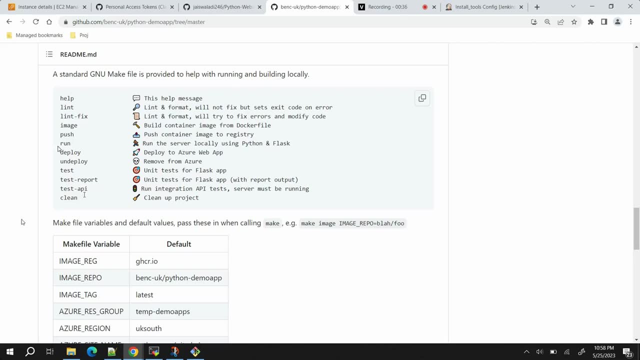 example, if i scroll down here, you can see these things. you are seeing. these are rules. for example, if i run the also like to run like make file command, we run, we type the command as make and the name of the rule. for example, we have this test. okay, so in case we want to perform test cases, we 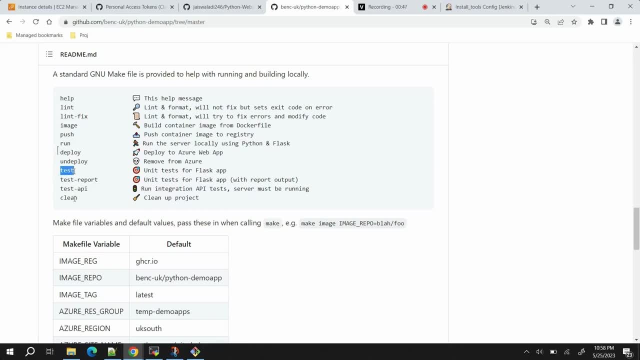 will run the command as make. then the rule name is test, okay. similar to that: if you want to clean up the project, make clean and but in in like. for our case, we will be using two of the rules, which is image and push. so using image, we will be building our docker image and using push, we will be pushing. 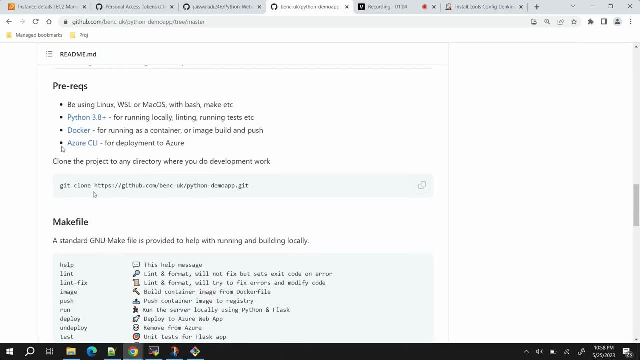 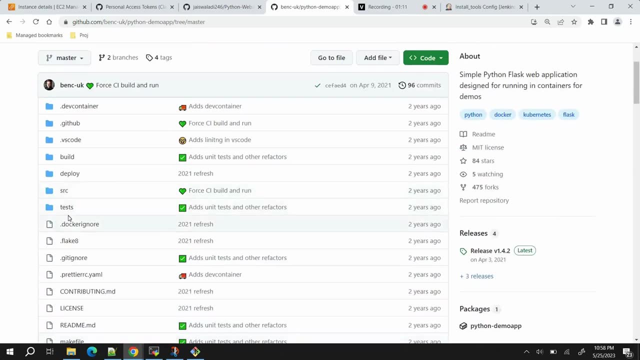 that docker image to our docker hub repository. okay, okay, now. okay. also one more thing, like, as i mentioned that, why this project won't be running if you directly clone and run the project in the same way. so this is the reason for that. there are certain. what is that there are? 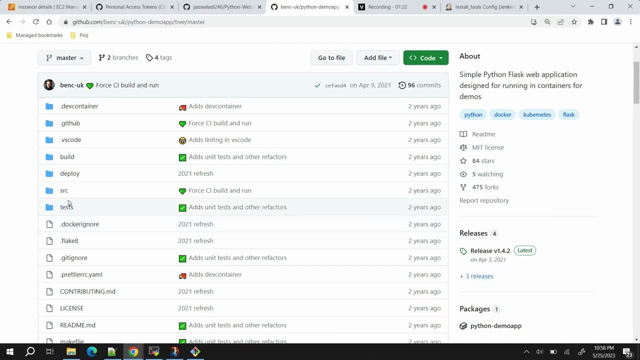 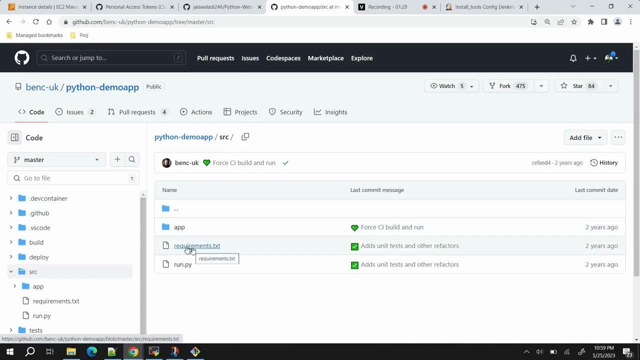 certain packages that are depreciated and they don't. they don't exist anymore. okay, so to fix that, first of all, what we will do, we will go to src. inside it we have one file, requirements dot txt. okay, so this files basically contains the list of packages which we are going to use in our project. 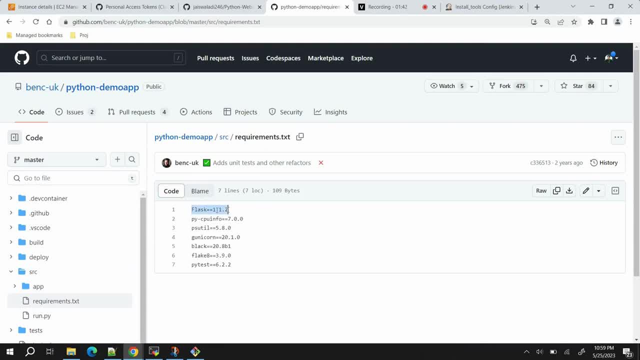 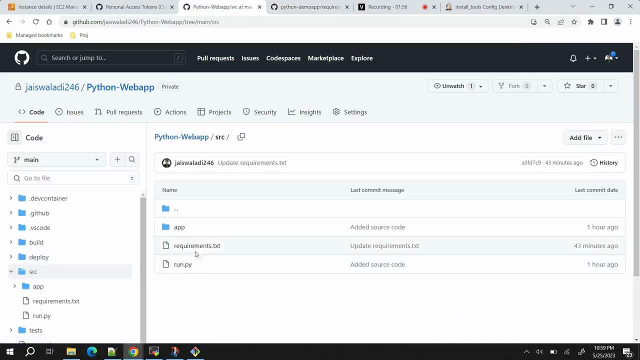 we can see so many are, so many of them are there, but, most important one, that we need to make changes is the flask current version. you can see it says 1.1.2. okay, so we need to basically edit this file and make the flask version. what we need to uh the changes that we will be making- is like we need to. 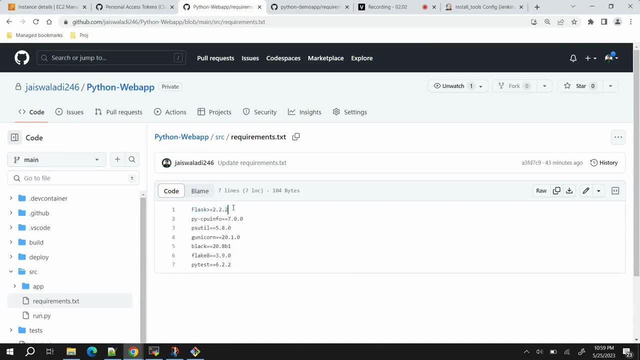 have this version. okay, flask greater than equal to 2.2.2: okay, this version, first of all, this version. if there is this version, then only our project will be able to run, okay, okay. also, make sure that you are basically forking this, uh, this one, which I will be sharing it, sharing to you, so fork it. 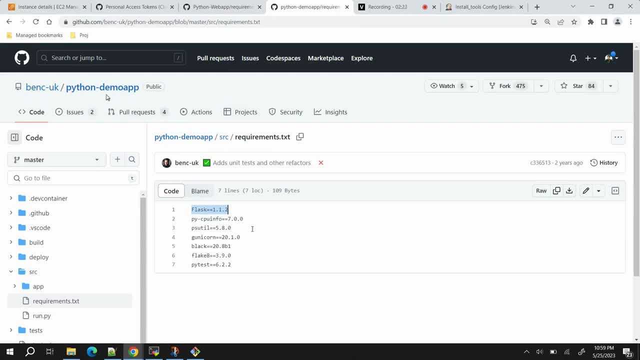 first in your repository, then only make the changes. the reason for that I will just explain you in a bit, okay, so first, changes that you need to make is in requirementstxt. what exactly is this file? this file contains the specific version of different packages that we need to have in our 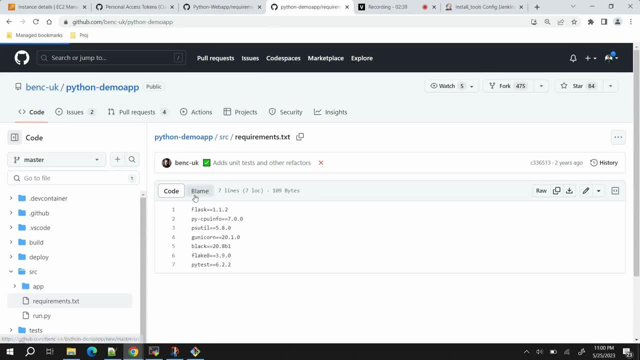 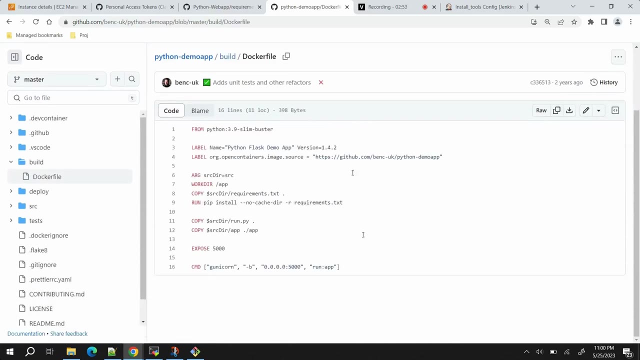 project. okay, so I hope you understand first part coming next: yeah, so we need to basically edit our docker file as well. you can see docker file exists inside uh project name slash build inside docker file. so let me open docker file and let me explain you what things we need to change here. we just need to change one. 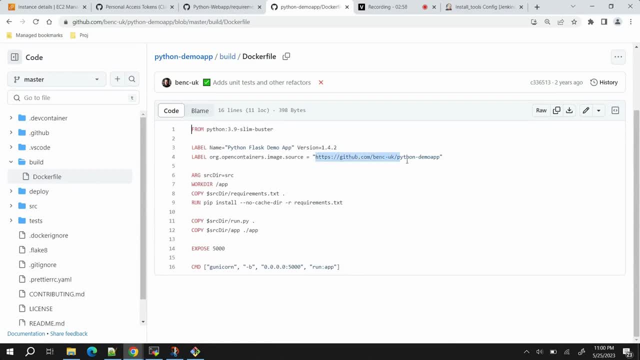 thing here you can see like directly, it's cloning the repository. so here, like, when you are cloning the repository or forking the repository on your account, then like, provide the your repository URL here, okay, because if you don't, then it will again. will it will again fetching all the. 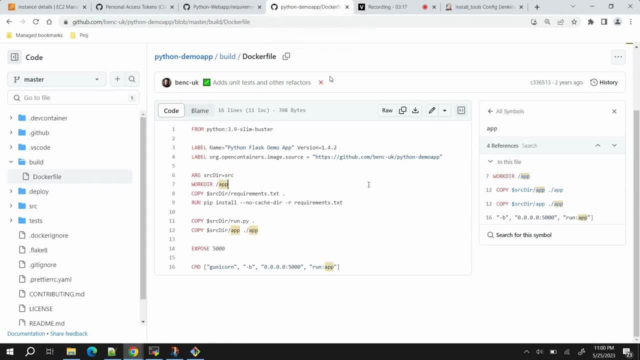 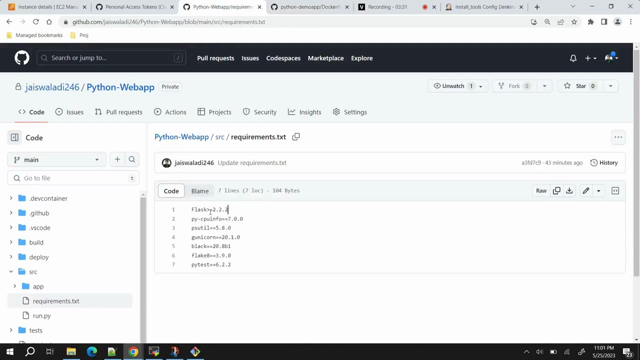 like uh repository and files from the original uh repo, and if that happens, then again all the flash question and every changes that you have made on your repository doesn't matter, okay, so make sure that you are changing this also. same thing like: let me just show you see, in my requirement: 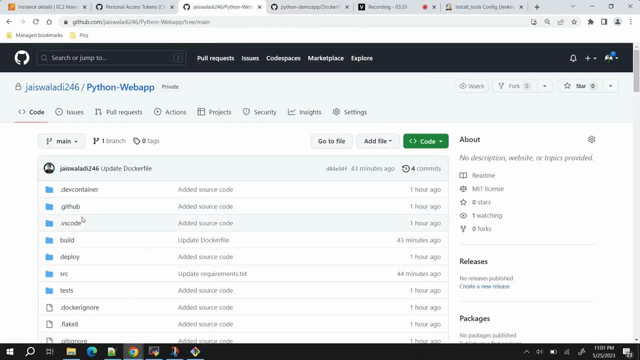 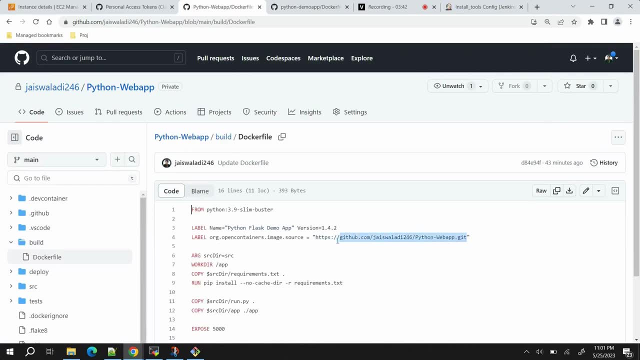 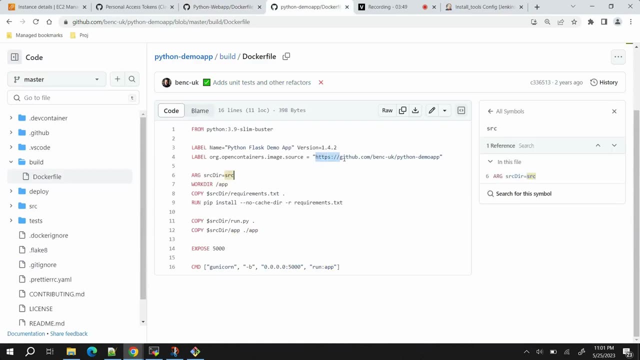 txt flask is this one, and if I go to build, let me go to build in build. we have docker file, so here you can see I have provided mine, okay, okay, so this is done. uh, also, like you see, make sure that when you are providing the URL, it should. 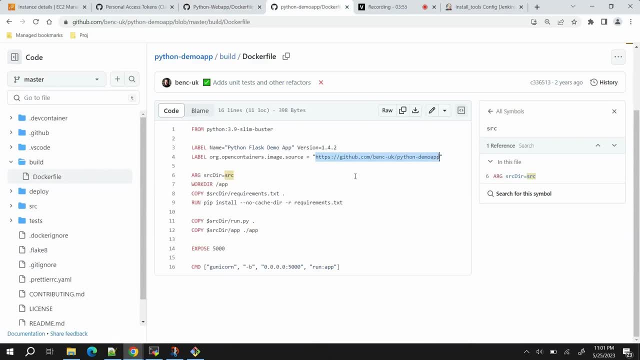 be public, then only it should be it. this docker file will be able to fetch it properly. okay, rest of the things you can see. like project is supposed to run on 5000, so 5000 ports should be open on your Ubuntu machine and this is the default command to run the application. okay, so these. 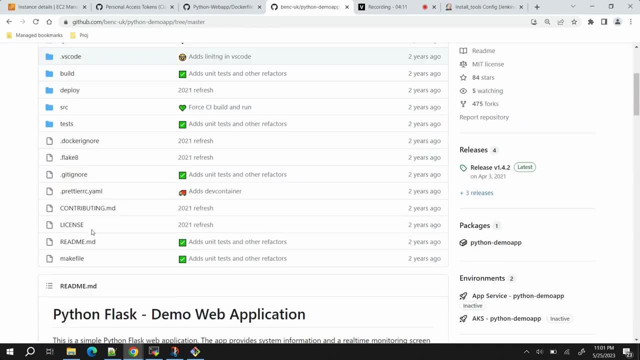 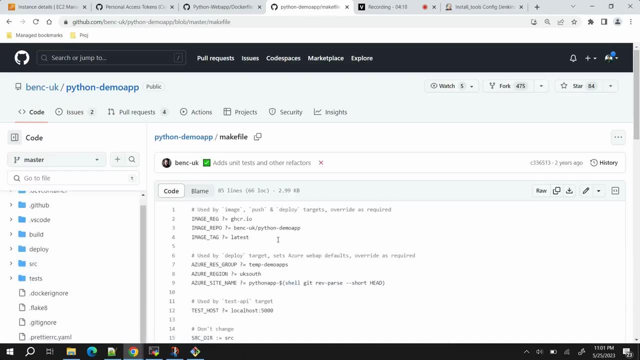 things you are done, okay. next thing: what we need to do is, uh, we need to make changes to it, okay, so, as I mentioned that, we are going to build the docker image and push it on our docker of repository, so you can see, these are some of the variables that are being used in your project. 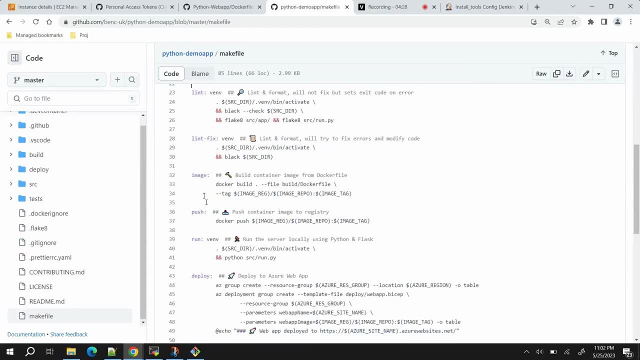 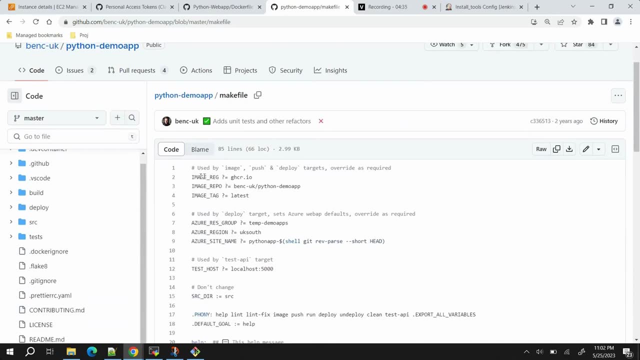 and downside we have the rules, okay. so, as I mentioned, two of the main rules that we are going to use is image and push, okay, okay. so in image section, first of all, we have image registry, basically reg is short for registry as per, and here you can see the registry name is: 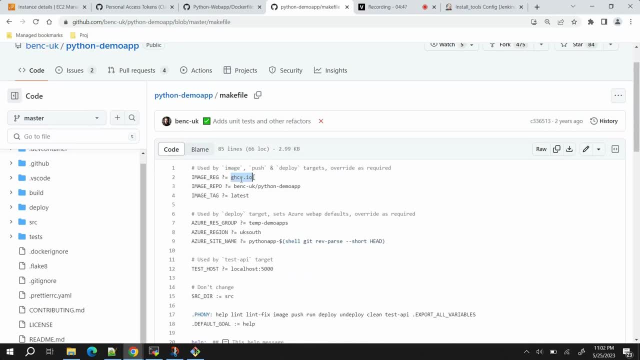 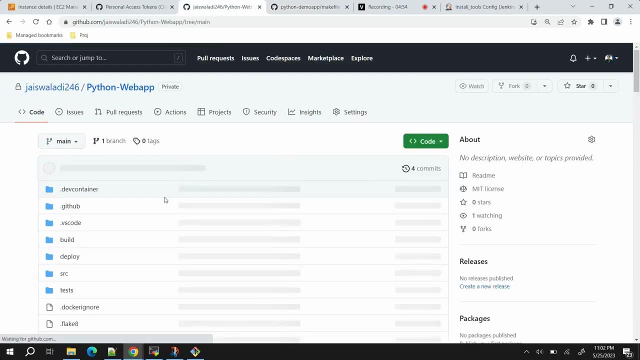 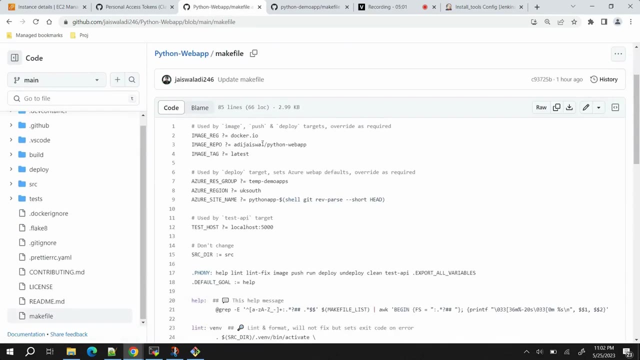 different because the owner of this repository was using a different registry. okay, so here what we need to do: we need to make changes and we need to make it a dockerio because we are going to use a public repository. okay, so, if I open, uh, my my thing, yeah, here you can see dockerio I have. 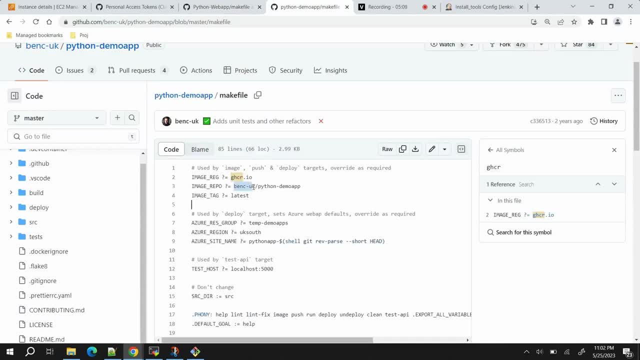 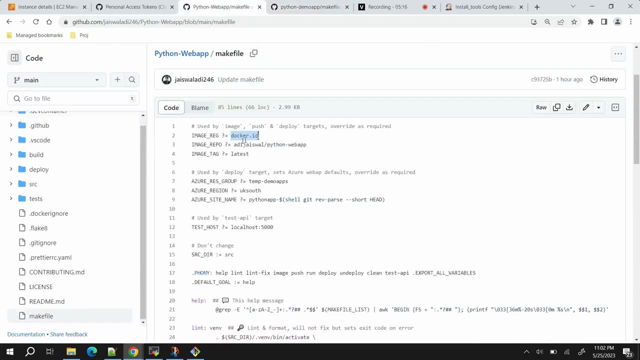 added next image repo. okay, so if you see here, as, as I mentioned, always like, first is the username name you want. so since we are going to use dockerio, the public docker repository, so we will provide our username, slash the name that we want. image tag: that will be same latest. okay, rest. 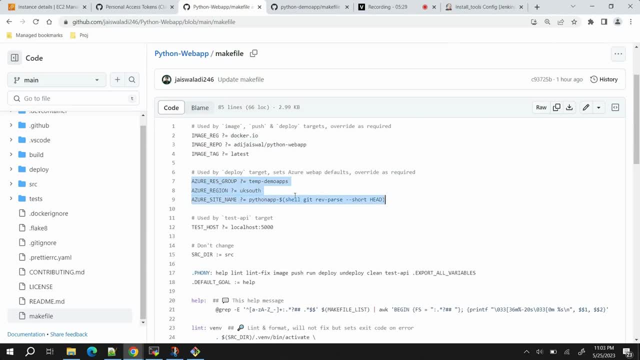 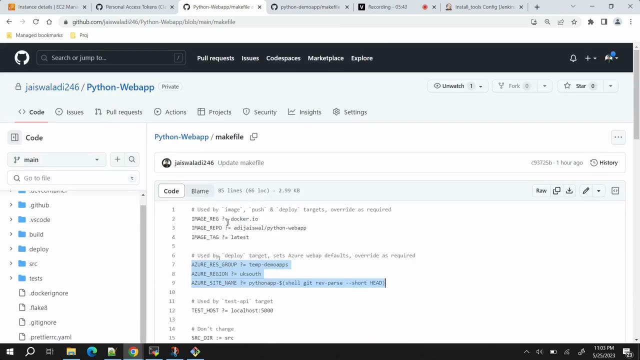 like in case you are doing, going to deploy this on Azure, then these changes, these things will be requiring changes. okay, but as of now, we are just going to deploy our application using docker image and docker container. okay, so rest to. I think I don't need to do any more changes. 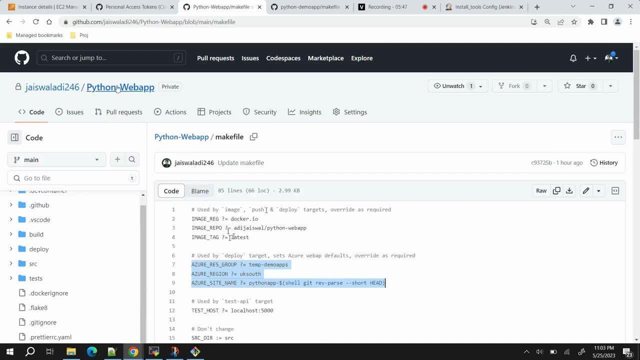 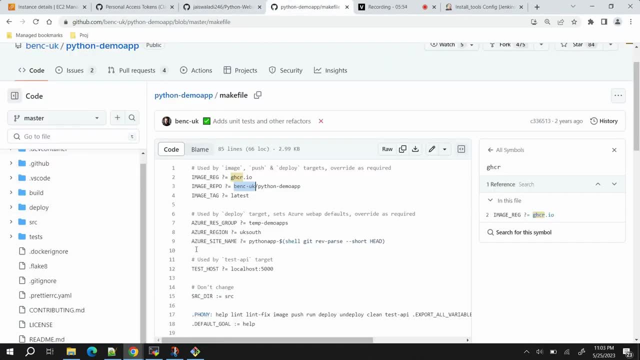 but these things you need to like properly change as per your credentials, okay, okay, so this is done. now coming to, yeah, this much changes only required. okay, these changes you need to make and I hope you understand at this point, like what is what exactly is make file? 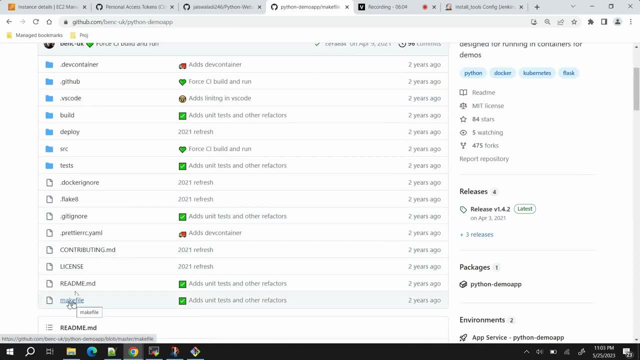 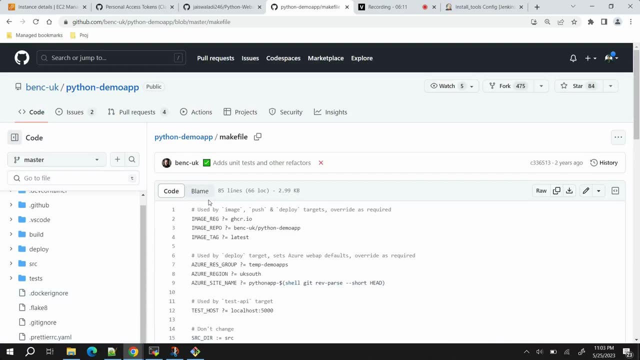 requirement- requirementstxt file. these two are very important files, okay, that that are going to be used for deployment and building. okay, just to show you again: make file is basically a file or a script which contains different set of rules, as different set of rules because of, due to which? 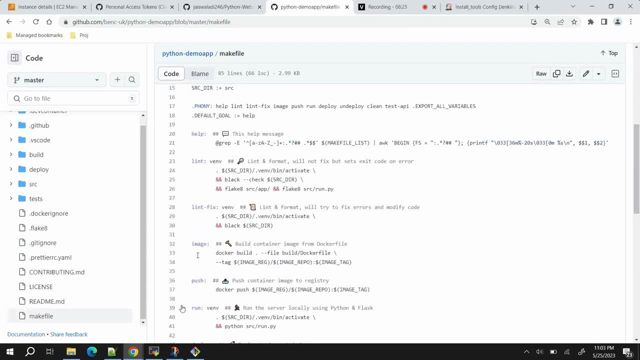 our applications, we perform different tasks, okay. so, as I mentioned, these are the rules: push image lint, fix lint, okay. so whatever we mentioned, whatever command we run that is like make lint, then that that will be happen. make image, then image will be building, okay. so these kind of 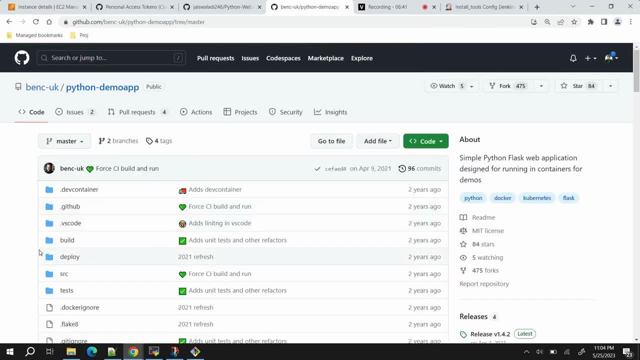 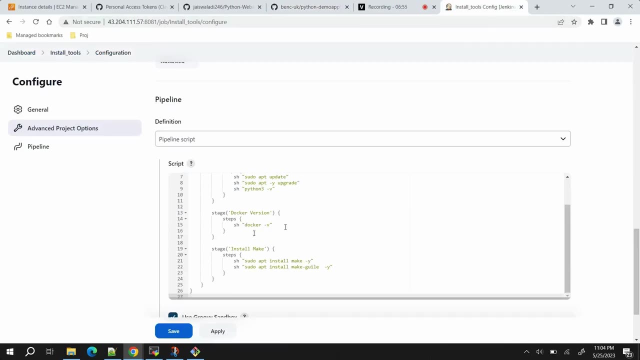 things will be happening okay. so I I hope you understood, like these are the things that you need to make changes. OK, so that is why, like, I'll be sharing you this URL so you can make changes and do your deployment, OK, OK, So, once this part is completed, what we need to do, we need to make sure that certain tools are installed on our Jenkins also. 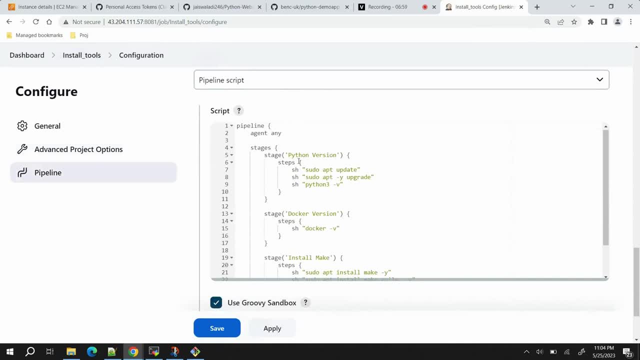 OK, so if I see I have created just one pipeline job for installing different tools, So Python. basically it might be coming in your Ubuntu machine or any other VM by default only, But just to make sure I have run these two commands: sudo apt- update and sudo apt- hyphen y upgrade. 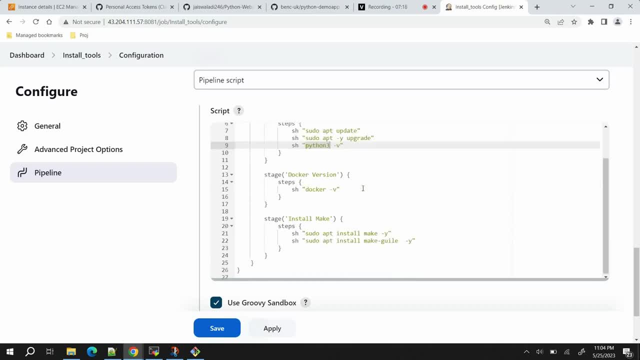 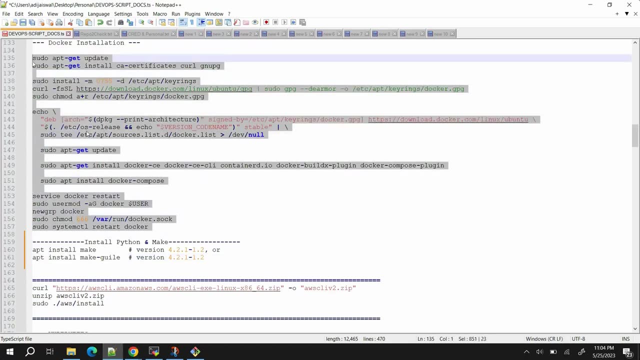 OK, then just to check the Python version, I have run this command, Python 3, hyphen v. OK, then Docker. like Docker commands I have already shared to you, like these are the Docker commands. OK, so these are already available to you, I guess. So you can just install them and then Docker version. 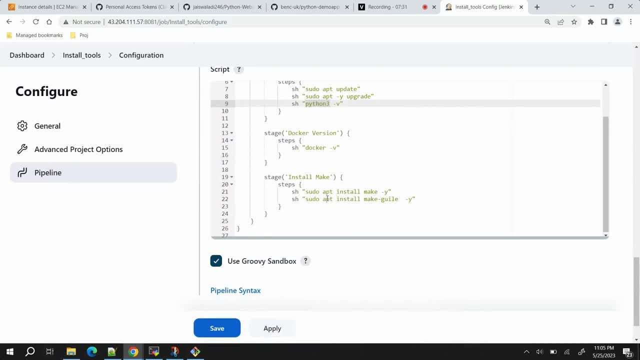 I'm just checking here. Next, most important, as I mentioned, we are using make file for building and deployment, So you need to install these make also, OK, and these commands also. I will just link in the description so you can install. 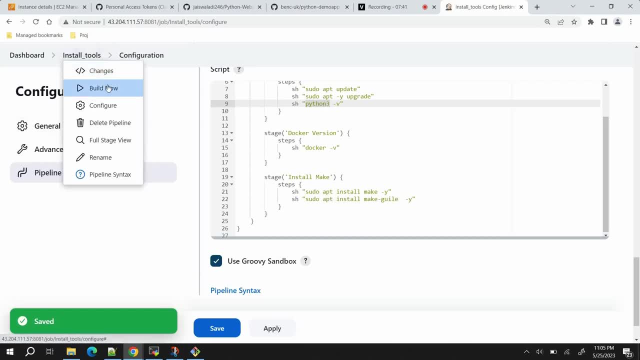 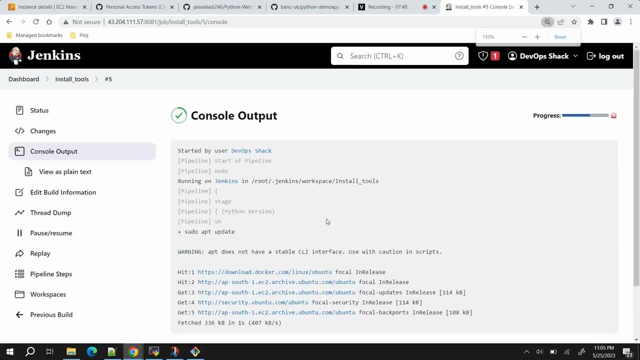 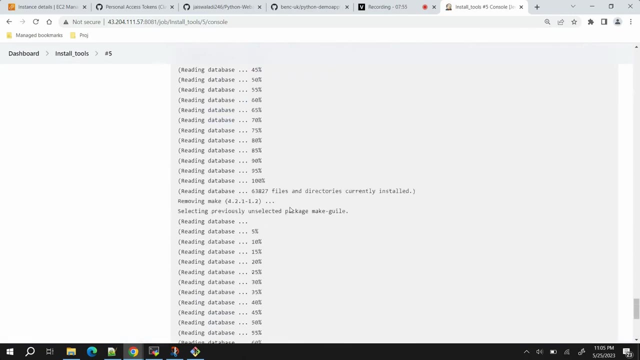 OK, so if I save this and if I I run this, these tools should be installed. We can track the progress here. We make it a little bit, Yeah, So you can see Docker version. I'm using the latest one, which is twenty four point zero point one. 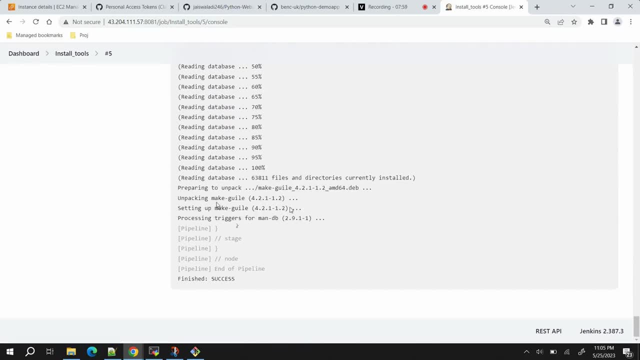 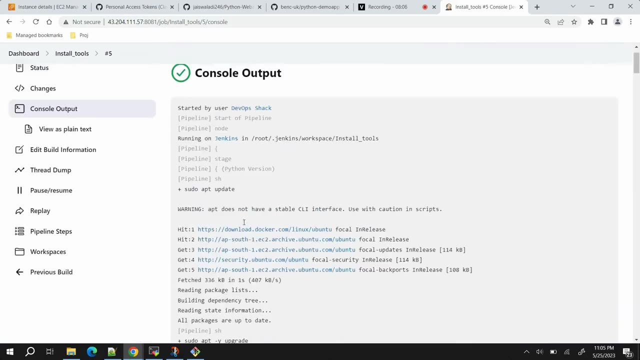 OK, and here it is. It has installed make also both. the make one is one is like, not make one is make good. OK, and Python is already installed. Python, which version I have, Let me just show. OK, so where is it? 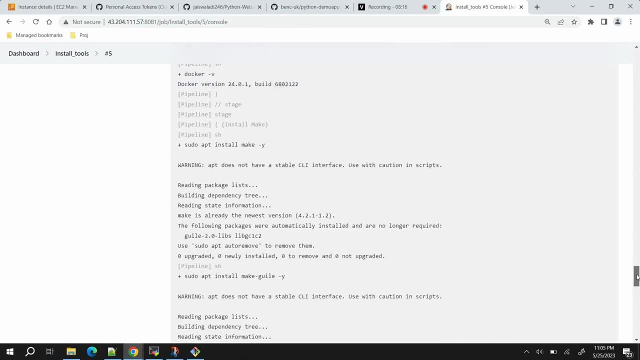 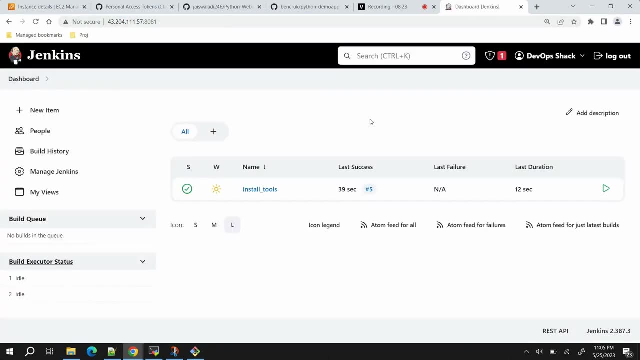 Yeah, OK, Python is already all already installed. OK, so, these things done, now what we can do, we can start creating our pipeline. OK, so make sure to still follow, because still I don't know what error will come, So let's just see. OK, so, OK, team. so basically, one more tool needs to be installed. 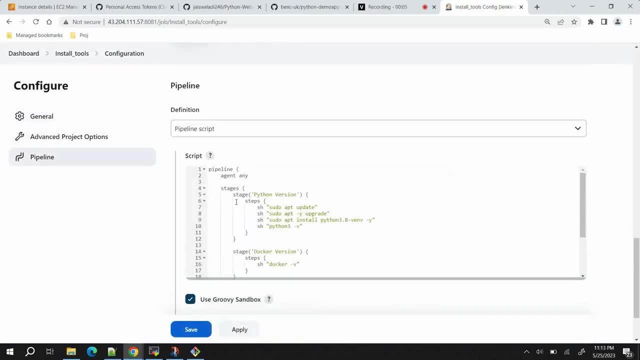 Let me just show you Also, like I will just mention all the things in description, These things Also need to be installed. OK, so make sure that you have installed Python as well as Python three point eight. We in Envy. 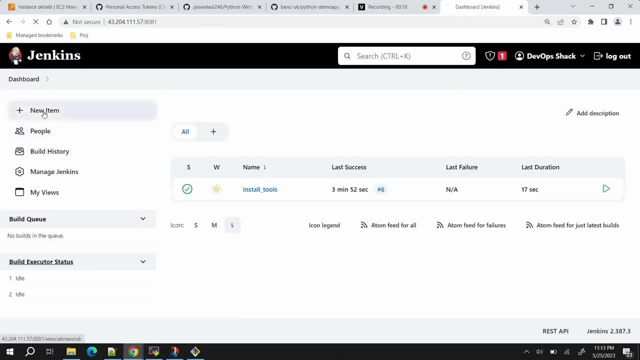 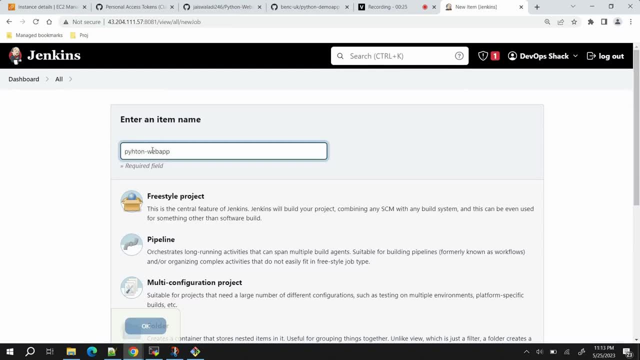 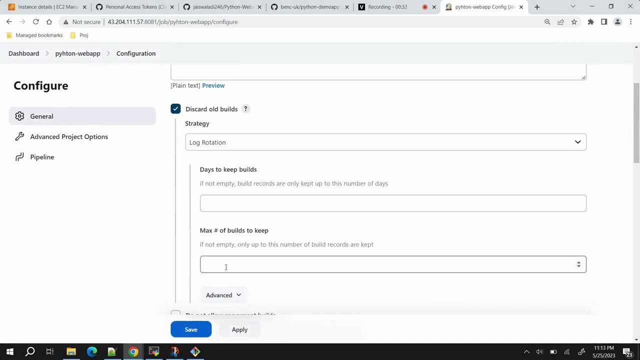 OK and make So this one should be fine. OK, now what we can do. we can create our main pipeline. OK. so name: I want it as Python Dash Web App and format type will be declarative pipeline Here. we will just keep as one this time and scroll down here. 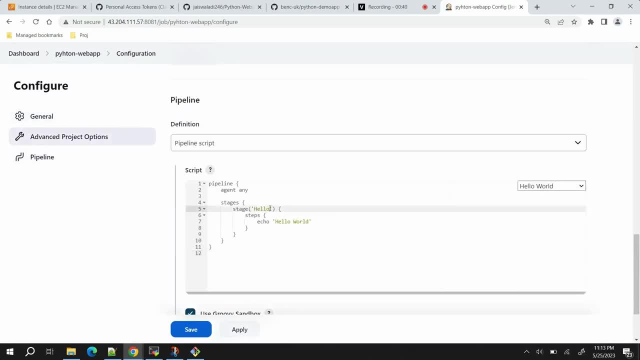 Let's generate a sample. OK, so we have one. OK, yeah, Also, this time, like I won't be like compiling or like performance on our cube checks, because this project already took a lot of time from me. OK, so we will just go straight to the point. 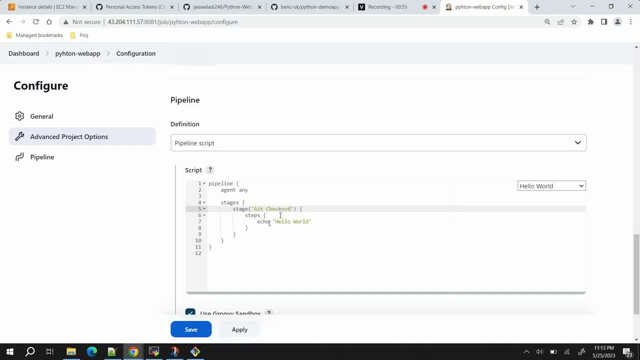 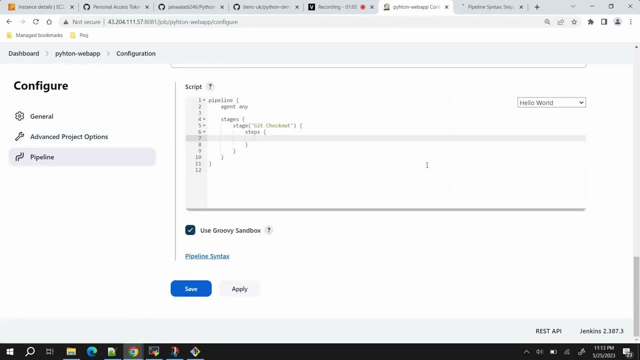 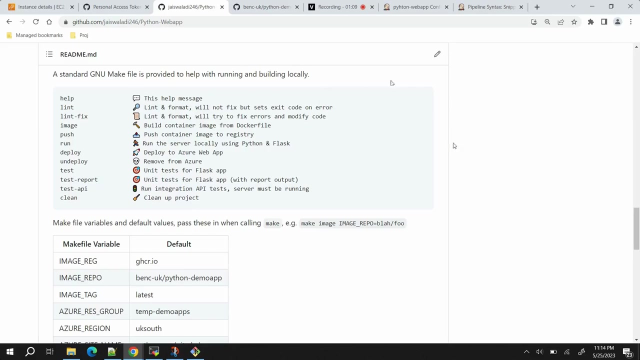 OK. so first we'll be having good checkout And in steps we need to provide the GitHub repository URL. so we will be using pipeline syntax as usual. Here we'll select Git And here we need to Report the URL. OK, so repository. 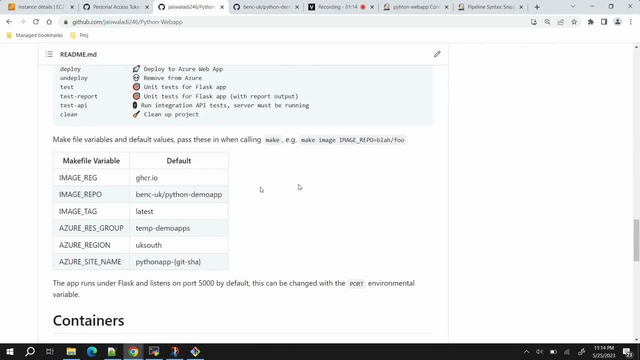 I saw one more thing I forgot to tell you. like in case, like you are having using a different image registry and repository, you can pass it in this format. OK, but for me I had just hardcoded all those things in directly inside the make file so that I don't need to make changes again and again. 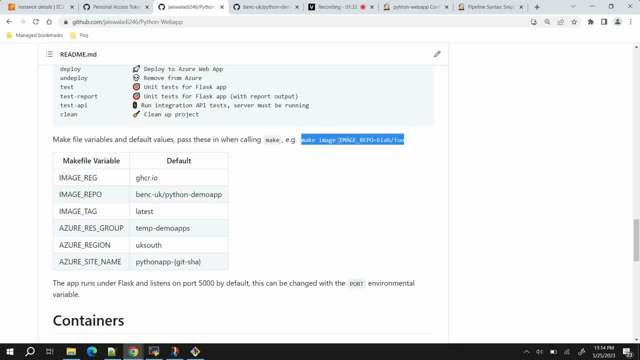 So either thing you can do, either make either like hardcode all the details, all the variables in your make file, or else you can pass these like On runtime. OK, Either is fine. OK, Yeah, So here we need to work the repository. 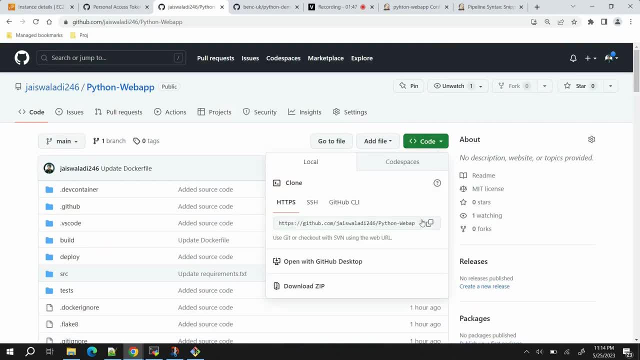 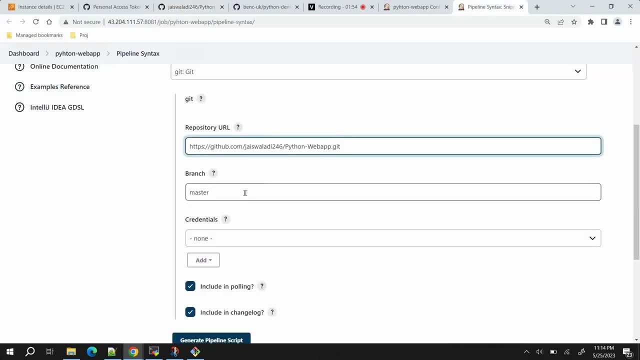 Let me copy the repository from here And paste it. Branch name is. Let me check. I mean: OK, No issues Branch name. We have configured as of now. I just kept it public, So we will. We don't need to put the credentials. 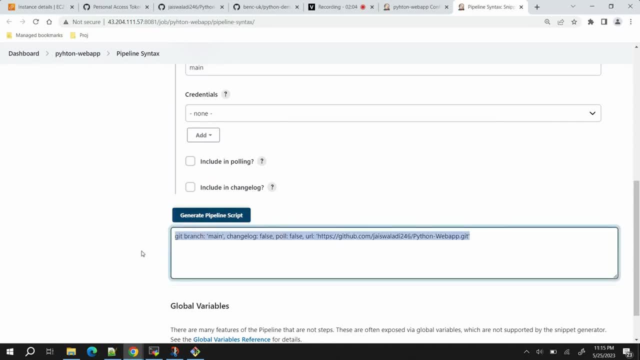 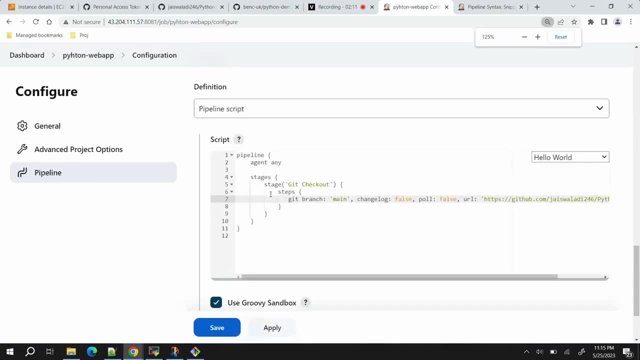 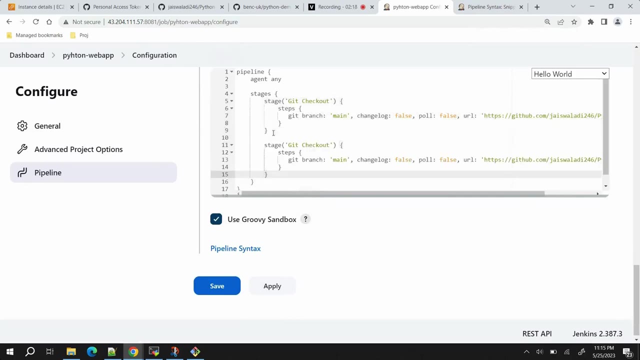 And let's copy this Copied And here we will paste it. OK, OK, OK, And here we will paste it. OK, This is done. So next step that we want to run is Build the Docker image. OK, 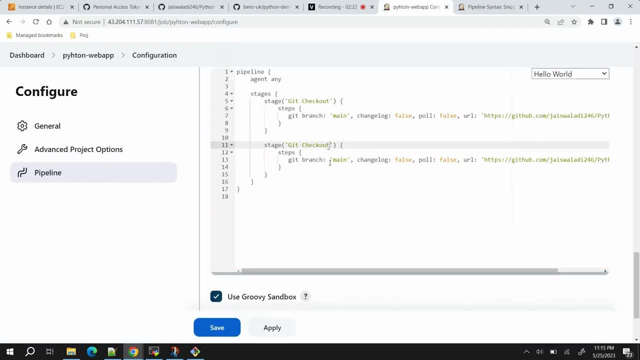 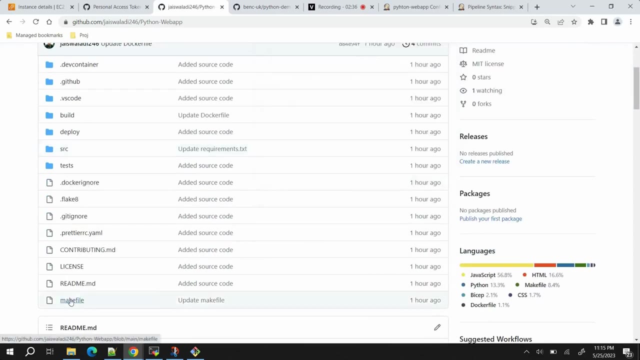 And let's- Let's provide a name as Docker build. OK, And all the commands that need to be followed is already inside our make file. Just to show you one more time, Let's open make file And Docker image rule. Yeah. 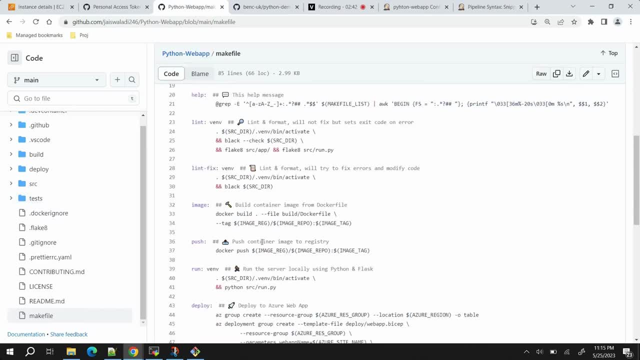 Here you can see Docker build And the path of the Docker file. Then we are tagging it as well At the same time. OK, OK, And See A command. Let me write it. Yeah, Here we can write the command as SS. 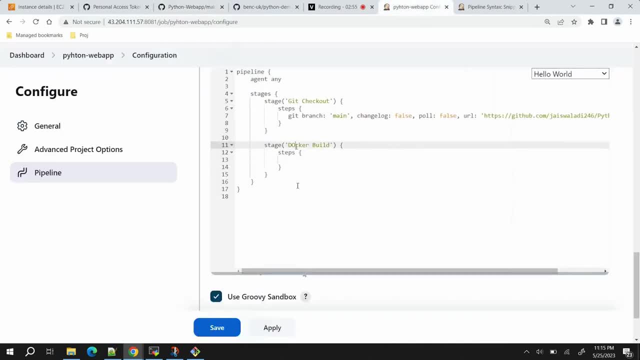 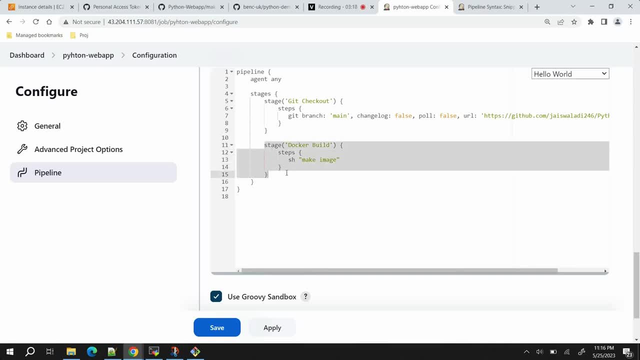 It will build the Docker image. OK, So, Side by side, What we can do, We can copy and write our second command, Okay, Which is to Docker push. OK. Now, The problem with Docker push is That it 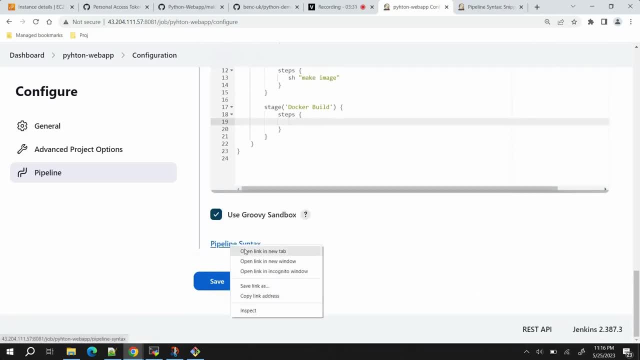 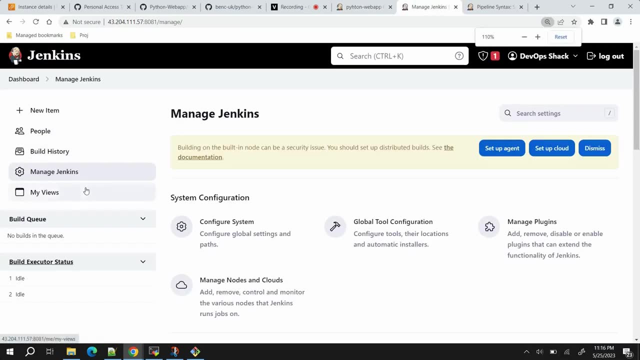 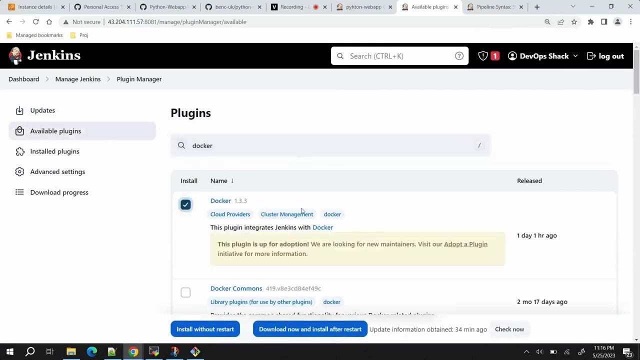 Requires credentials. Ok, So we need to first log in Then run. Run this command. OK, So what? I Will do that docker plug-in? okay, so we will go to manage Jenkins, go to manage plugins. in available plugins, search for docker and install without start. I think that. 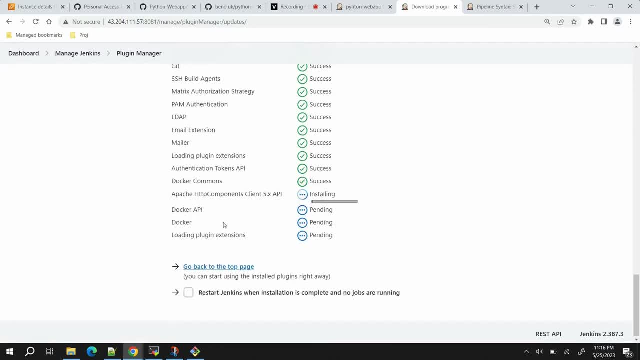 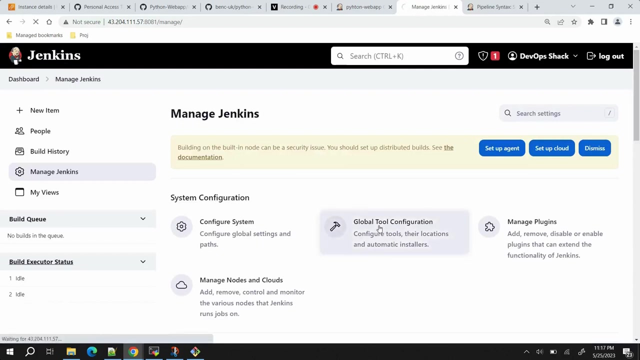 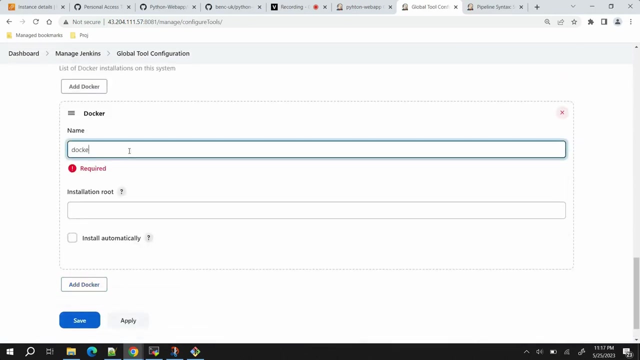 should be fine. okay, yeah, it's almost almost installed. let's see. yeah, so it's installed. what we can do, we can go to global tool configuration and configure our docker tool. okay, you can see, docker tool is available here. we can provide the name as docker installation automatically. we want to do from the official page of dockercom latest: 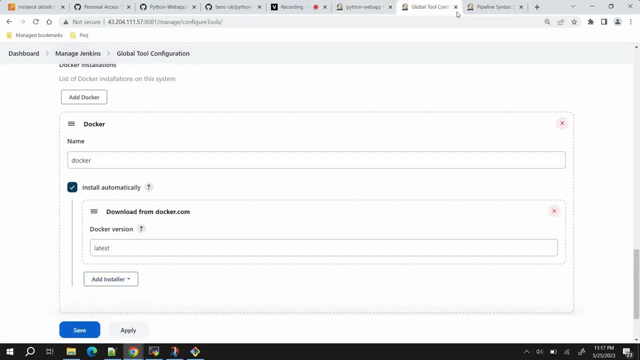 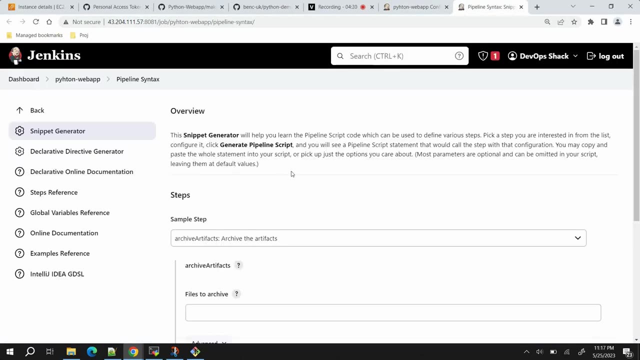 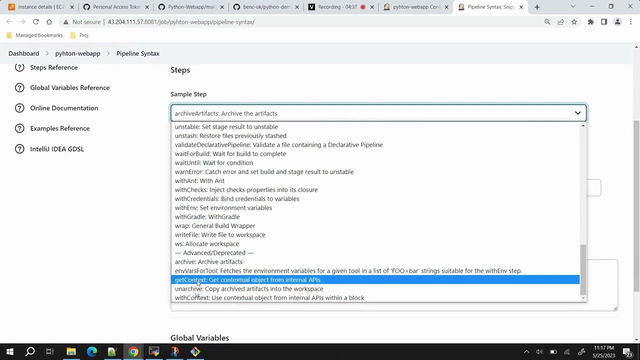 version we want, click on apply and this is done. so let's close this. yeah, so okay. so again, let's open pipeline syntax, and here we can create a script for ourselves. scroll down to with docker registry. see, here it's not available. the reason for that: we just installed. 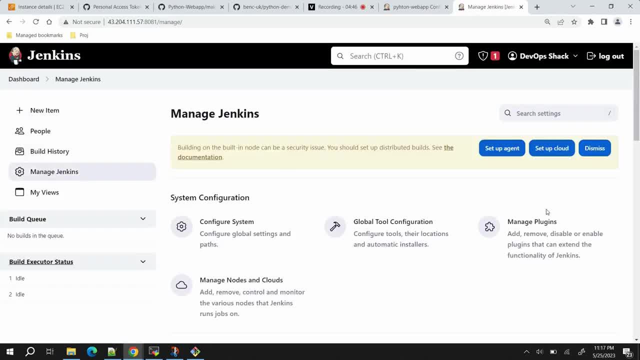 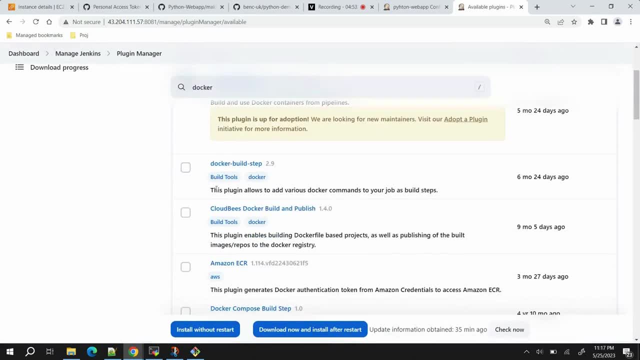 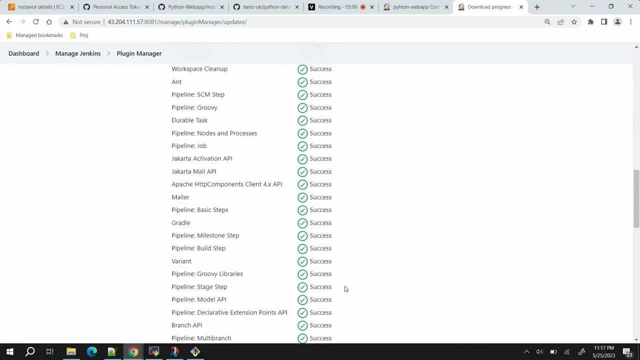 the docker tool. instead of that, we need to install few more plugins. so let's do that. and here again we'll search for docker. so docker pipeline, docker build step and these three, these three usually install so that I can like create the command and close the credentials inside a docker script. okay, meanwhile, we here also. 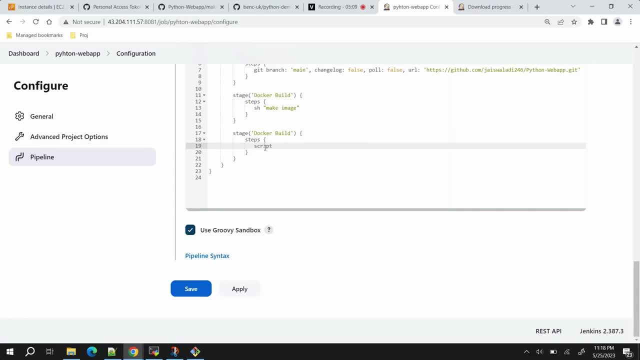 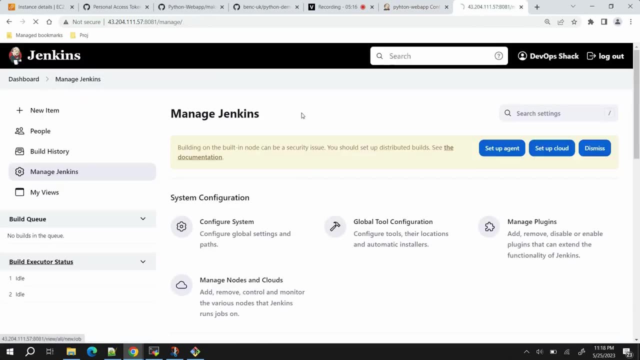 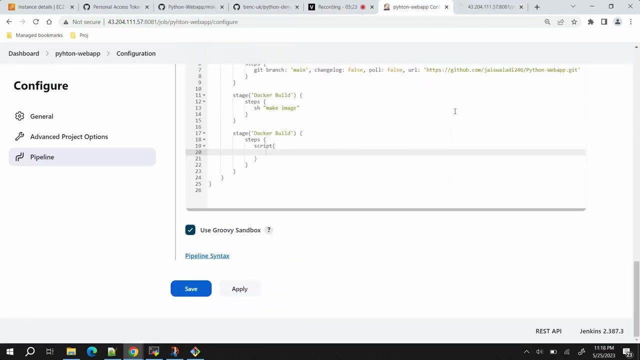 we need to create script. let me write it script curly braces, and inside this curly braces we will be writing our docker commands. yeah, so this. now it's been installed. let me close this. and now, if I open the pipeline syntax, we should be able to see that with a docker registry option. okay, we can. 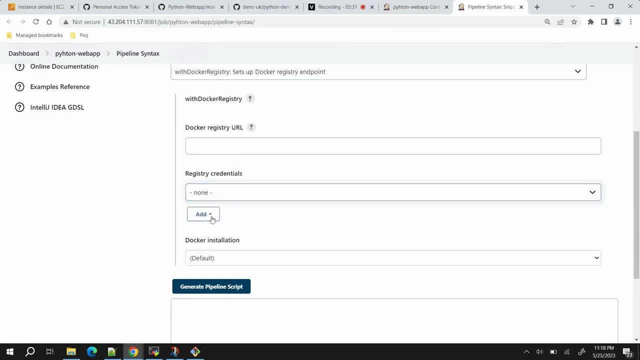 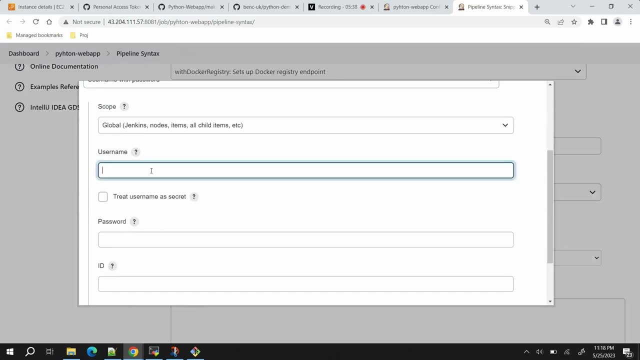 see it is available now. okay, so credentials. let's add credentials. see, the reason for adding the credential is that we need to push our docker image to our docker hub repository. okay, so username. let me check these. well, correct password would be this. let me just rewrite it. 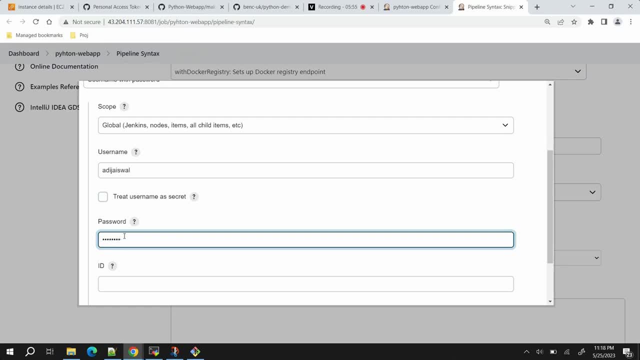 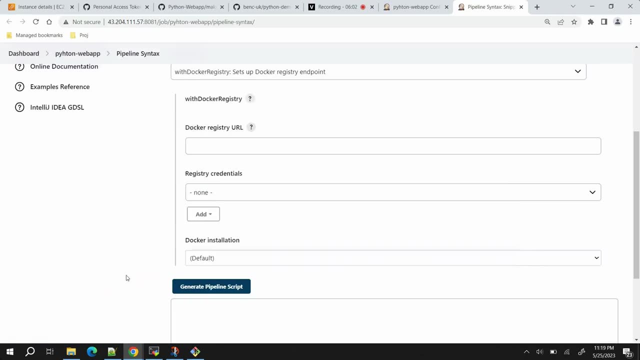 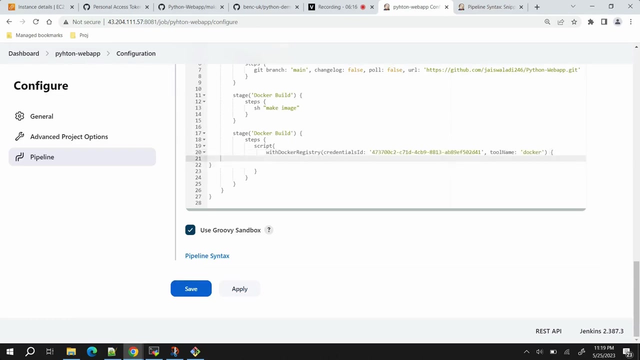 yeah, yeah, password also given now. last command is docker create. click on add. i hope you are watching because it needs to be done properly. okay, so this also we have created. we will paste it here. lets remove this command and align this braces. okay, so here we will run the make. 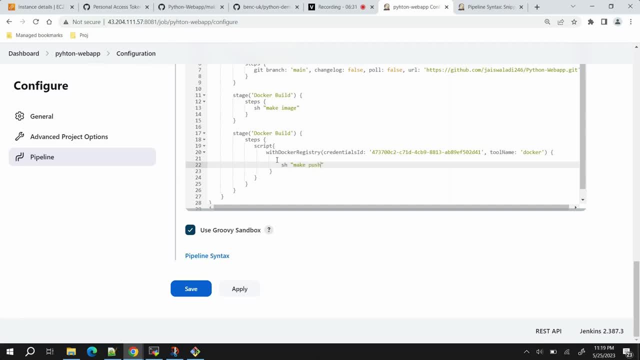 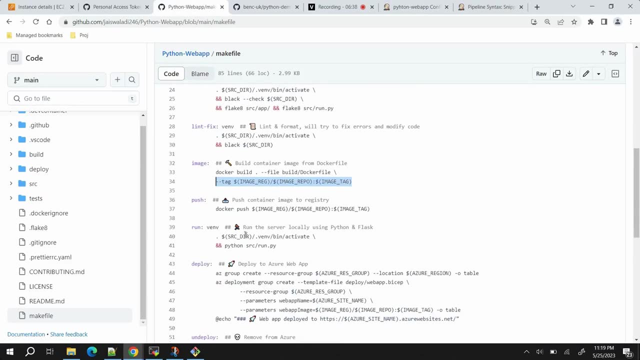 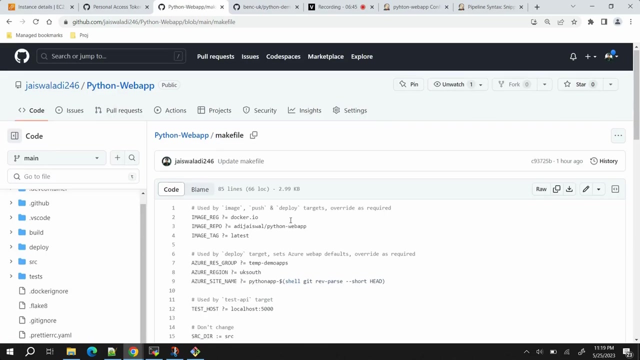 push command. okay, make push and this should be basically. see, i have not written any command for docker push. basically, if i go back here, you can see the command is already written and the details of image name, image registry and tag is already getting from the values that i provided here. okay, okay, so this is. 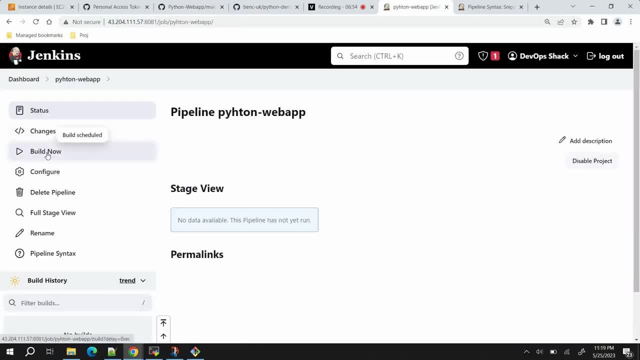 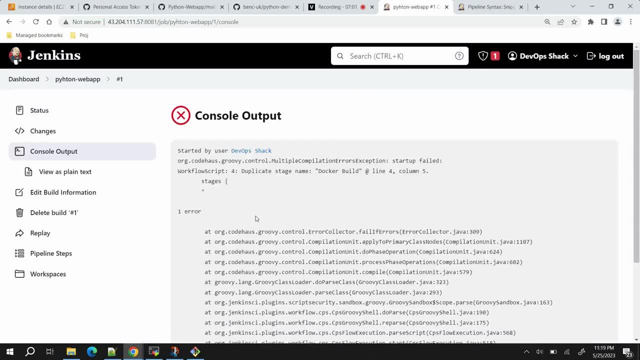 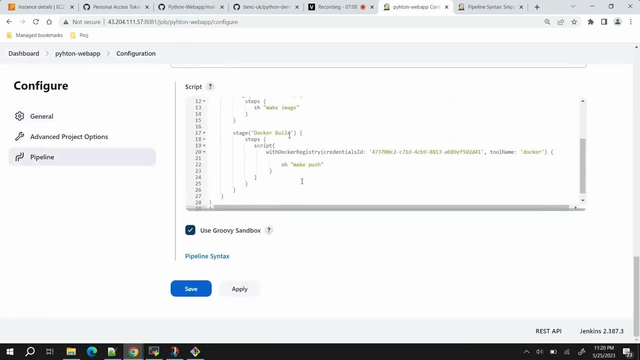 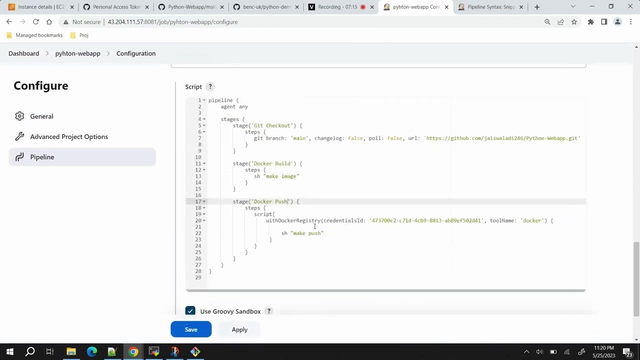 done. click on apply build now and let's see if it is able to do or not. okay, still, okay, it failed. also, no issues occur build? i think we have the two stages with the same name, i guess? yeah, see, i have always mentioned that whenever two stages are having same name, pipeline will fail. 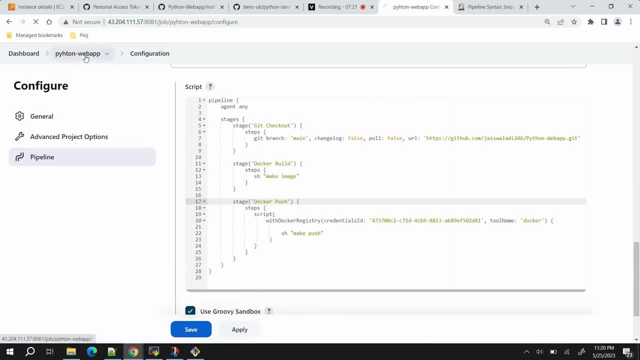 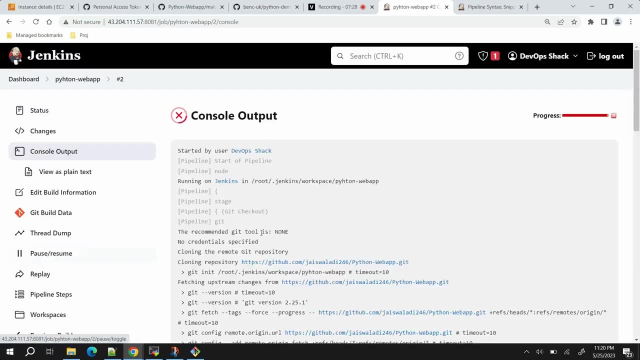 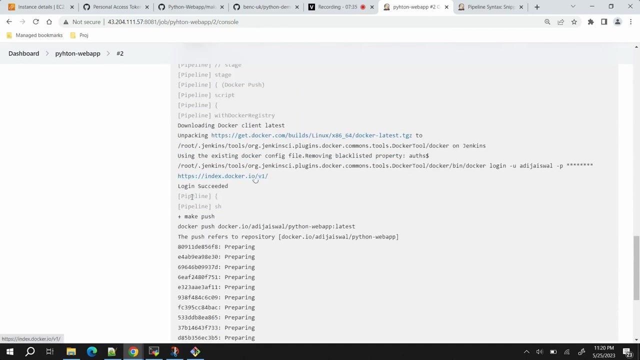 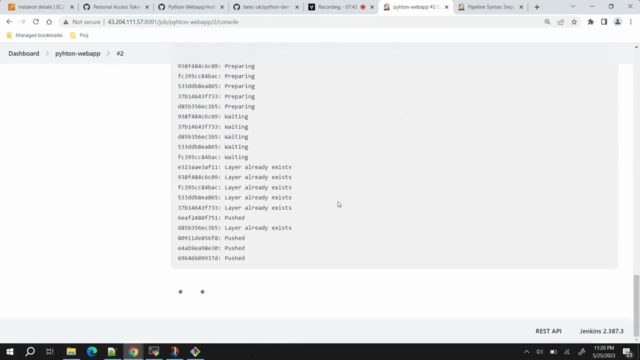 but stupidity is that even i forget sometimes. okay, we will build now again and let's see if it starts. yeah, so it has started cloning done. this one is creating the docker image done and it is able to see. as i mentioned, we need to provide the credentials so that it can. it can be able to push our docker image. okay. 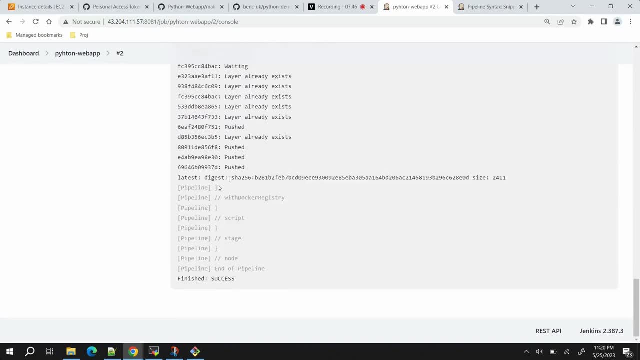 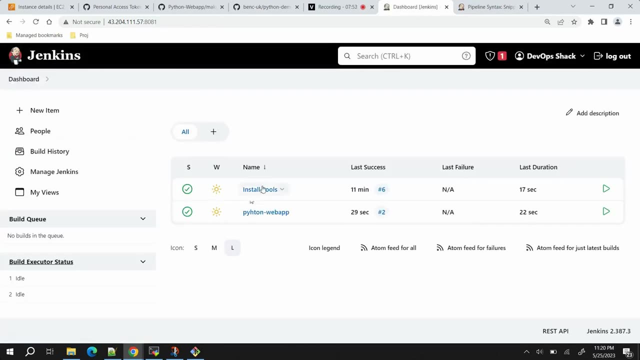 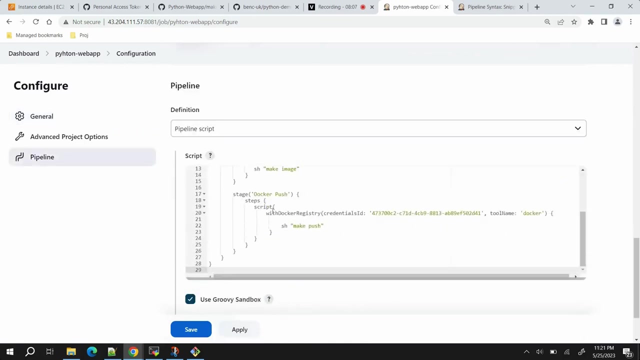 okay, yeah, you can see docker image is pushed if i run one command. let me sorry. i want to check the docker image name, okay. okay, side by side what we can do, we can directly deploy our application. okay, so if i open this, go to configure, scroll down here. this thing's done. 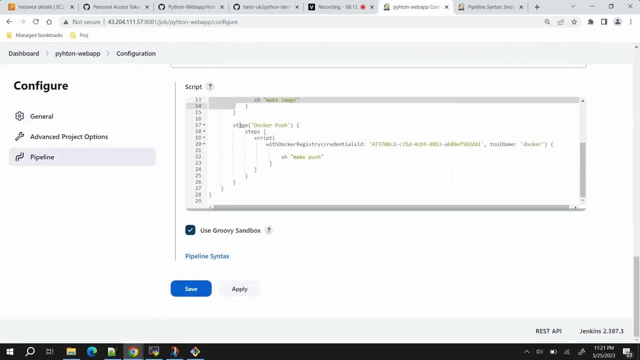 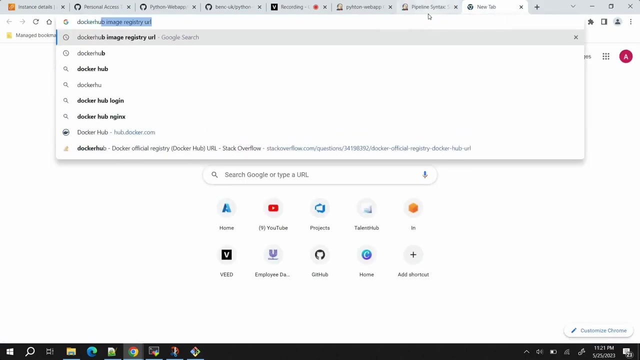 so i can again write the command for this. let's copy this, paste it here and here. we want to provide the details as docker deploy- okay, and the command that i want to run. first of all, basically, i want to check the image name- okay, docker images. and then we want to deploy it also to see that, if it is pushed successfully, we can go to go to docker. 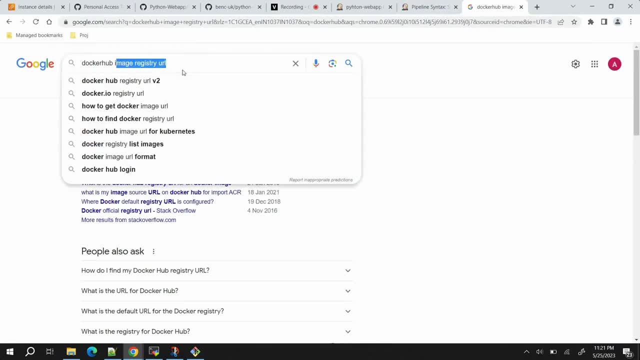 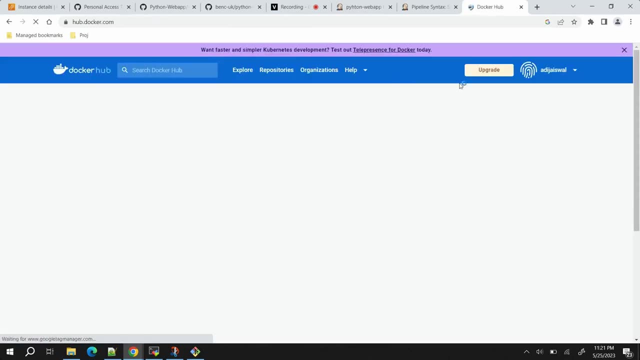 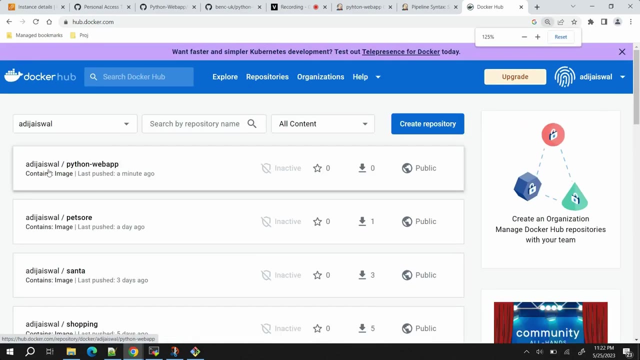 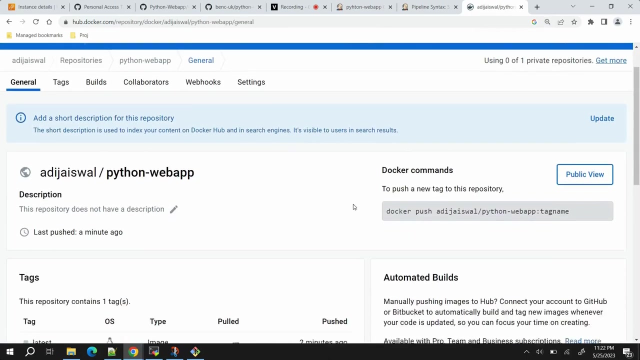 hub, okay, docker hub, and here we can log in and we can, we can be able to see our docker image. so if it exists, that means it is successfully pushed and then we can. okay, great, you can see here, if i zoom it a little bit as well- python dash web app. okay, so this has been pushed and we can copy the this one image, docker. 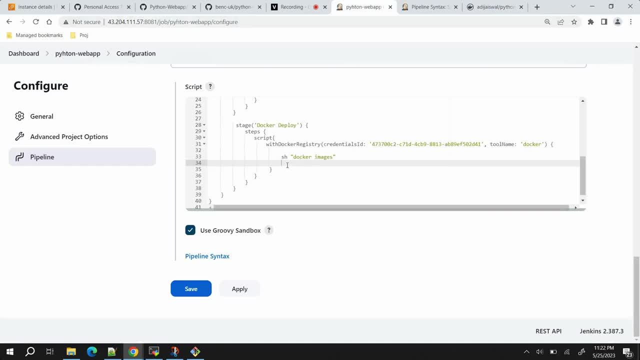 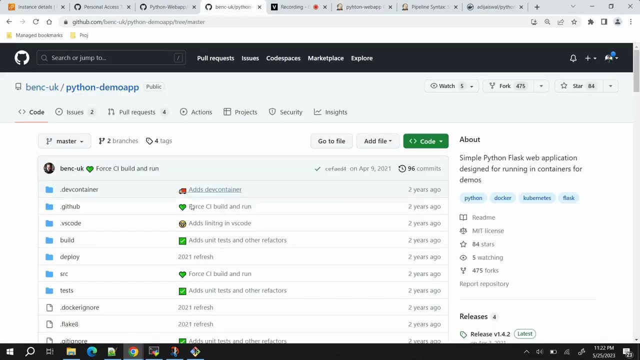 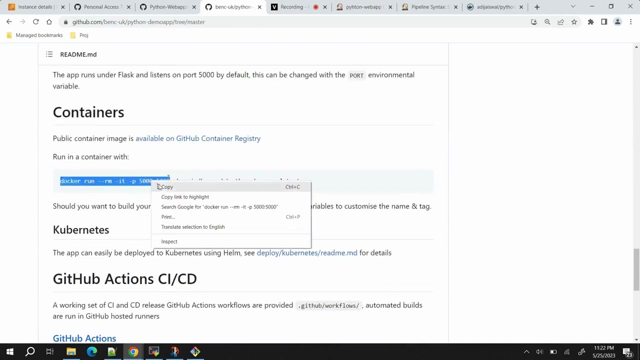 image name, okay, and here we can try to deploy, try to basically create a container, okay, okay. so the first command that we need to write let me show you: yeah, this the till, this must. you can copy: okay, prior task token: problem: docker imposed on the docker directory and then you can see it when i 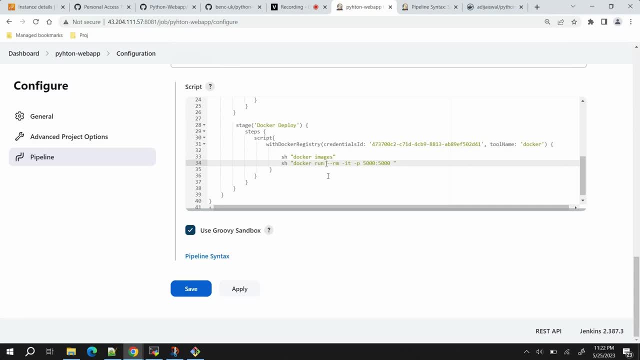 paste it here. okay, now what we need to do. first of all, make sure you are running it in hyphen d so that it runs in background and your job can finish. okay, because if you don't put hyphen d, your job keep running and like it won't be finishing. so that is a problem, problematic thing. 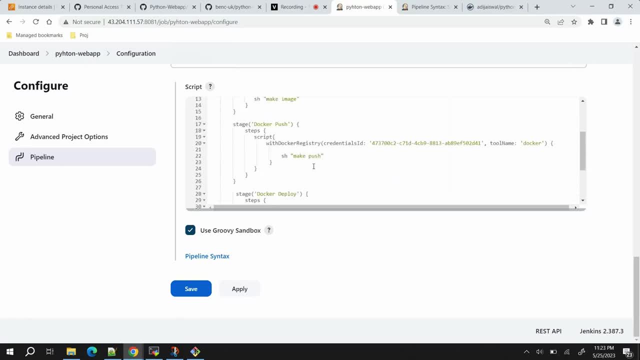 okay, and now we need to provide the image name here. tag we have is latest, okay, okay, i think this should be fine and it should be able to run. now. let's do the same mistake as well. so let's go back here now and go back to flavor page and stop. that's there. but that's nothing right? this one doesn't matter. 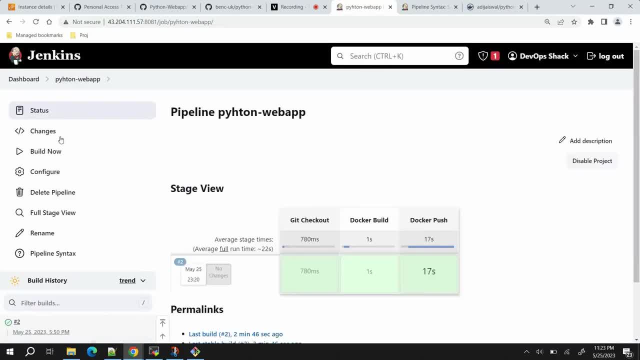 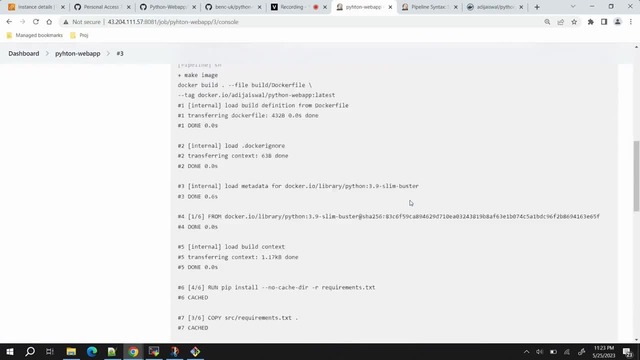 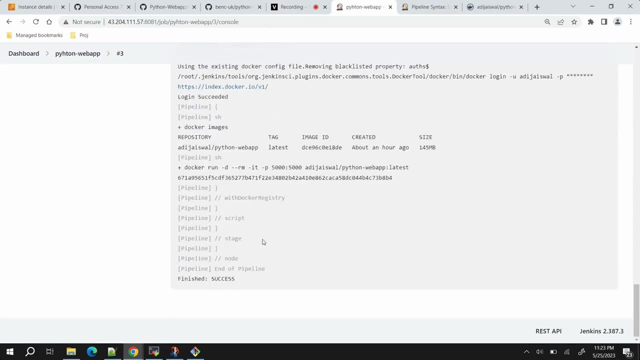 so we get hell of B, basta more like that. so this image that we need to run is kept like this for one minute to deploy our application inside a container. so let's do that. click on build. now progress. yeah, image build, it is being pushed. docker image pushed and now it is login succeeded.